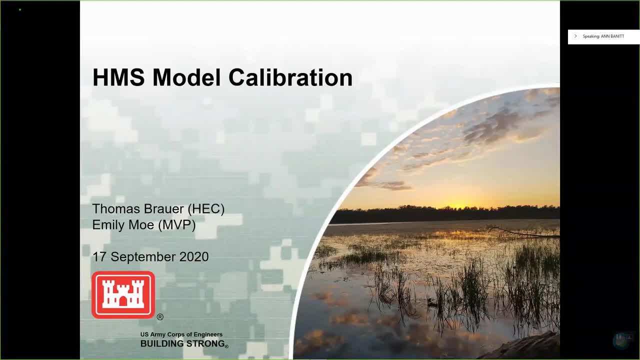 And I wanted to welcome everyone to the MVD Hydrologic Engineering, Statistics and Risk Sub-Cop webinar, and I want to welcome you all and I want to give a very special thanks to our speakers today for sharing with us some tips on HMS model calibration. The presentation is brought to you by Tom. 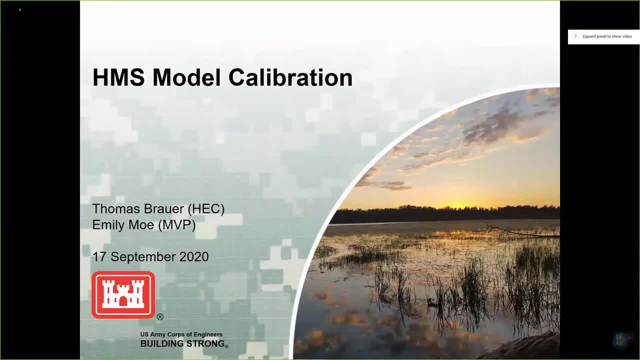 Strower from APC and Emily Moll from the Saint Paul District and I'm just going to give you a little briefing on on their backgrounds and also it's kind of the order. Tom's going to give you a little bit of front-end information that he usually gives at a HMS training class. 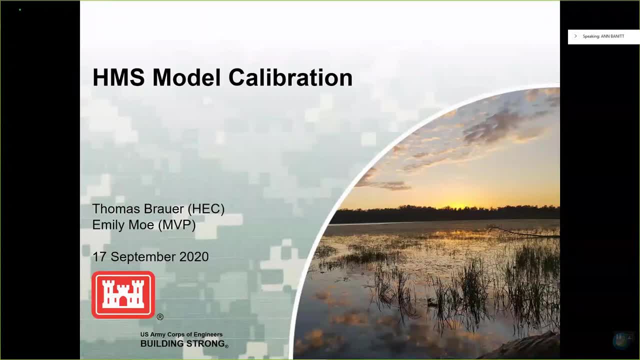 gives you some background on calibration. Emily's going to bring some more hands-on and specific tidbits from her work with HMS calibrations that she uses in teaching people to use HMS, especially on the swim side, and then it'll hop back to Greg to close things out and he'll give a little tip on some of the. 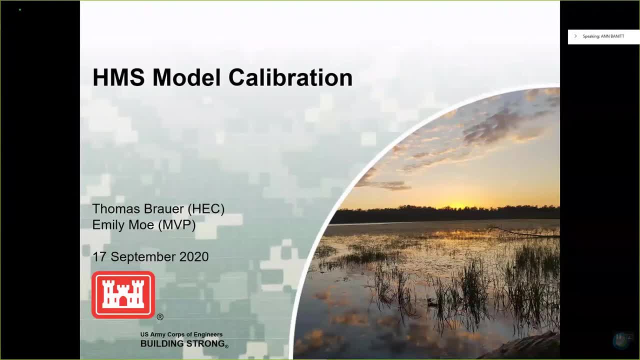 tools and tricks that are coming with HMS in the new version. All right, Tom is the lead developer on the HMS team at APC and gives a lot of these presentations in the APC training classes. Emily Moll: she is a senior hydraulic engineer at Saint Paul District and has really worked a lot with 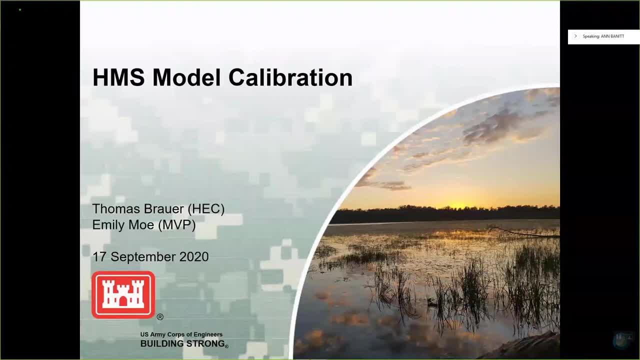 HMS development for the SWMS program does ADS modeling. so she's got an MDSA modeling and has a wide variety of modeling experience there. but she's able to really communicate clearly on the how-tos and makes it really understandable for people especially. 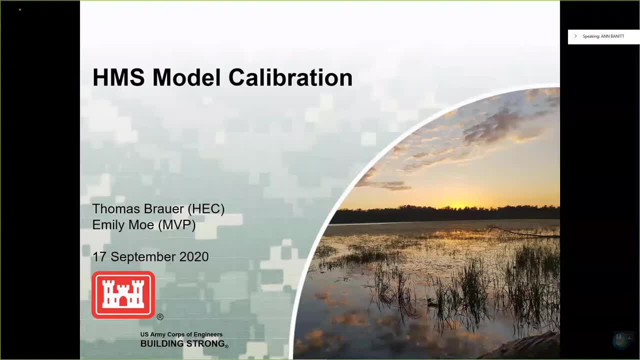 hopping onto these SWMS models that are brought to the district. With that, I'm going to turn it over to you, Tom, to take off with the presentation. All right, so just to check, you can hear me and you can see the slides. 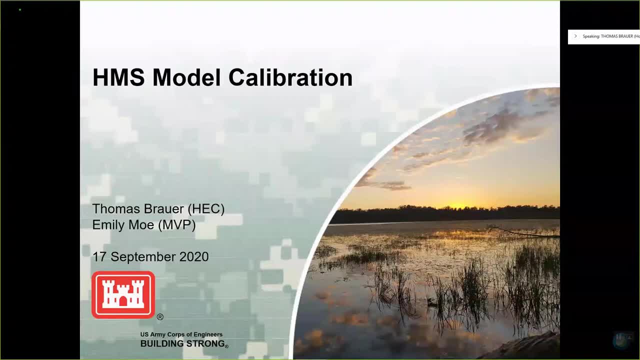 All right, I can hear you. All right, cool. Well then, we'll get rolling. I'm going to have, so here's my video now. see me while you can. I'm Tom Brower, and now I'm going to cut out the video. 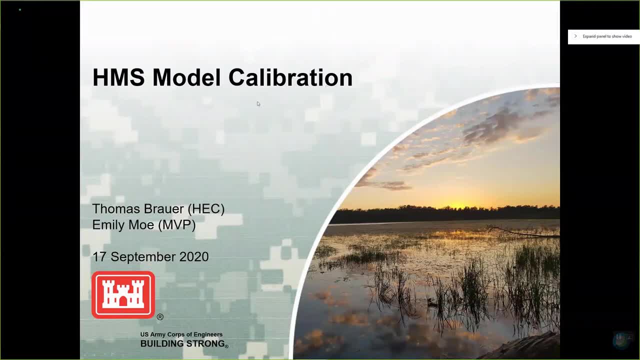 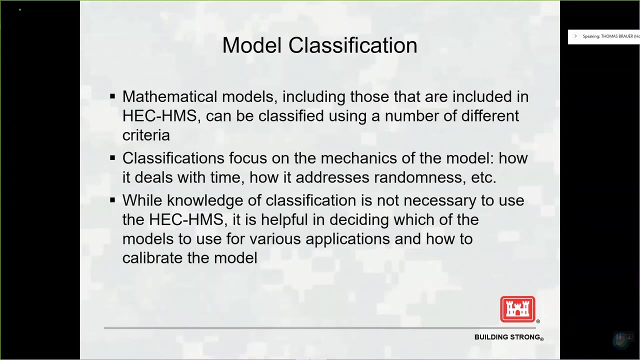 while I give the presentation, Okay, video off, And so we're going to talk a little bit about model calibration and, like Ann said, the first couple slides are going to be from our HMS basic training class, so you might have seen some of this before. A lot of this conversation is going to be in the context. 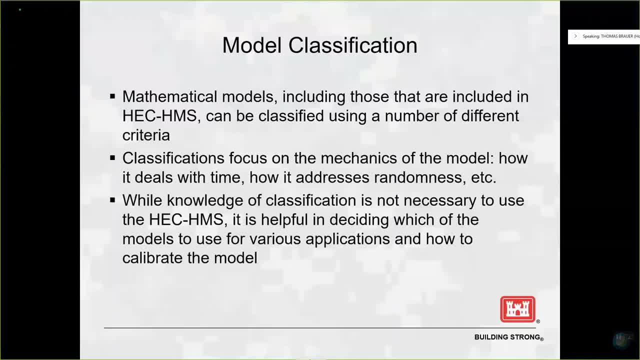 of real-time forecasting, so I'm going to try and tailor the content for that. We always start the lecture with a little bit of theory and model classification. I have to kind of minimize that based on time today, but there's a few things that are worth. 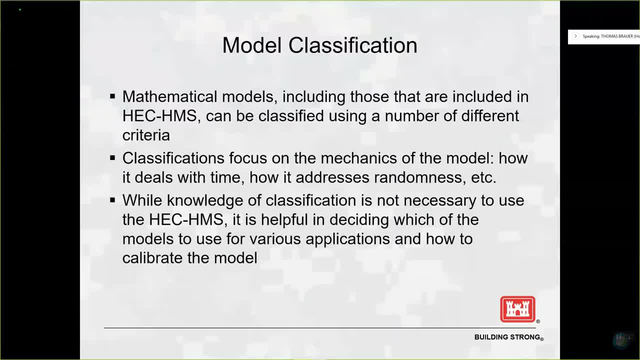 discussing, and so just a little bit on model classification. the mathematical models, like the ones used in HMS, to be classified in a number of ways, and well, you don't have to know the ins and outs of the different classifications to do modeling. it's helpful to know these for calibration and know like what. 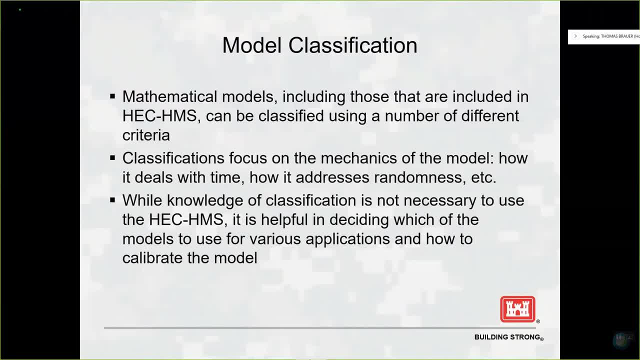 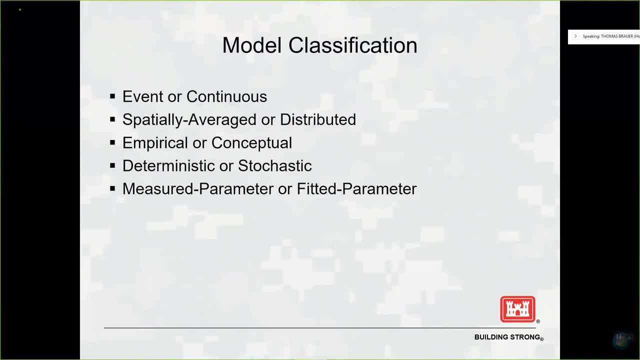 parameters you're changing and why you're changing them. so a little bit of knowledge of classification is important. here's some common classifications. reason modeling- and anytime you're in the modeling world you'll hear these terms- event and continuous is one. we'll talk about a fair amount today. spatially. 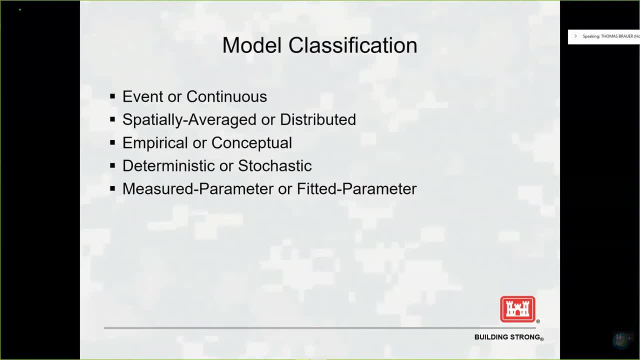 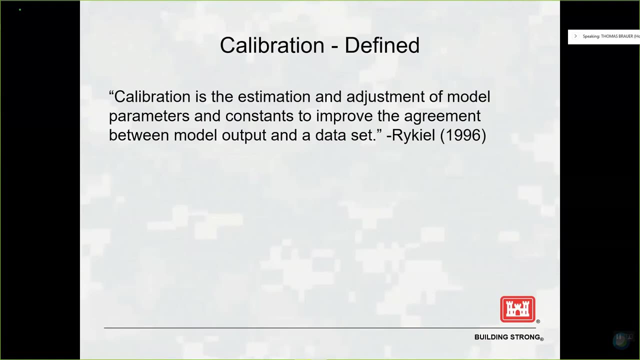 average and distributed. that's another way to classify: empirical or conceptual, deterministic or stochastic. this is a measurable measure, parameter or fitted parameters, another one we'll talk a little bit about today. so with that, let's talk about calibration. so calibration define. calibration is the estimation and adjustment of model parameters, and 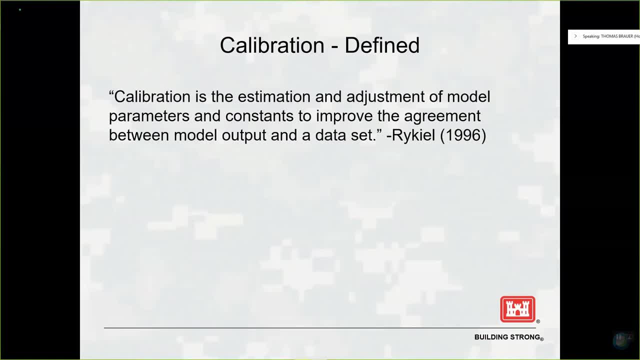 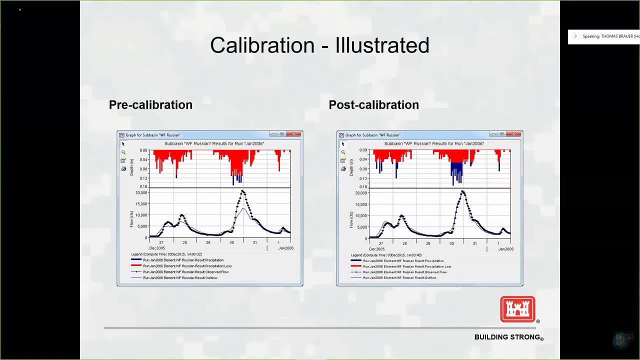 constants to approve the agreement between model output and the data set. so here's this calibration illustrated. you see, on the left pre calibration, the black line with little dots is our obscure flow, the blue line is our simulated flow and you can see that you know if the model is not performing. 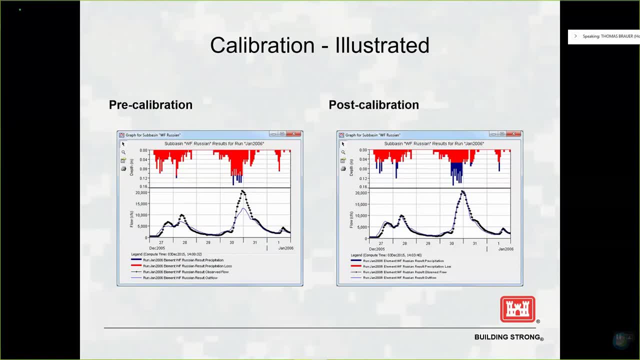 great, and so what we do is we calibrate the model to get better agreement between simulation observed. all models require training data. it doesn't matter whether it's a machine learning algorithm or an HMS process based model. so all we're really doing here in the calibration process is training a model on data set. 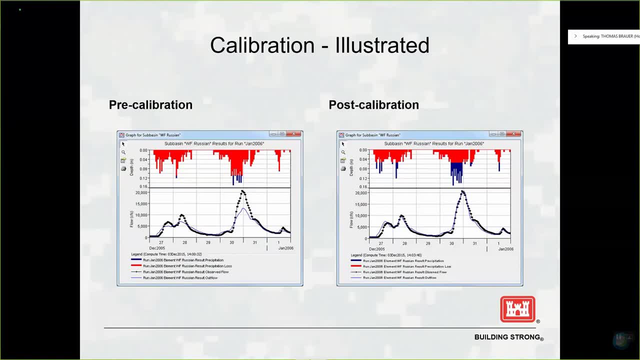 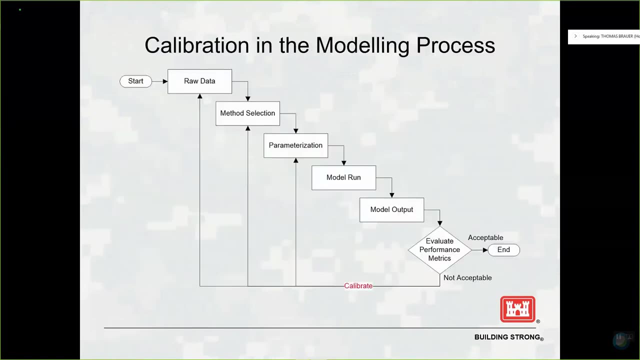 Now the hope with process-based models like HMS is that, because we have processes that we're modeling and physical processes that we're modeling is that we need less training, data Calibration and the modeling process. So this little flow diagram I just put together: 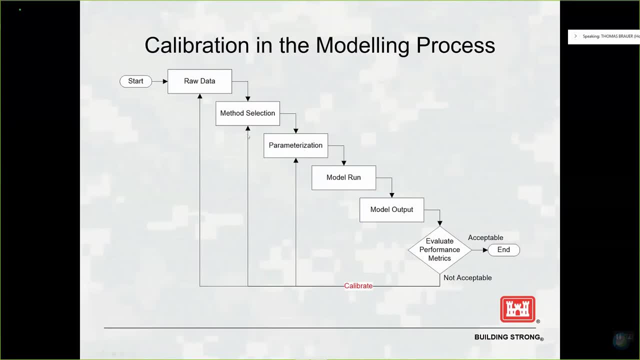 And so what most people think of when we talk calibration is this parameterization piece. So what I often want to do when I talk about calibration, and what I often see, is we need to come back around often and reconsider our data input, our raw data and our method selections. 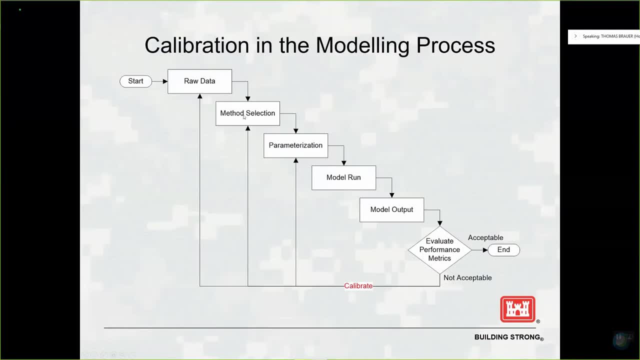 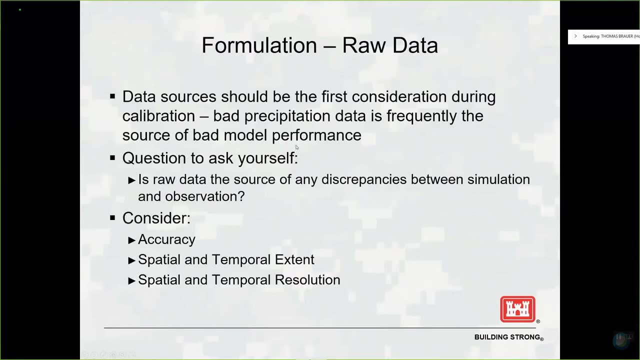 So, before you reconsider those if your model is not performing well, I wouldn't try to do this parameterization stuff, So let's just talk a little bit about that. So this would be considered. the model formulation is data gathering, but I think we should consider 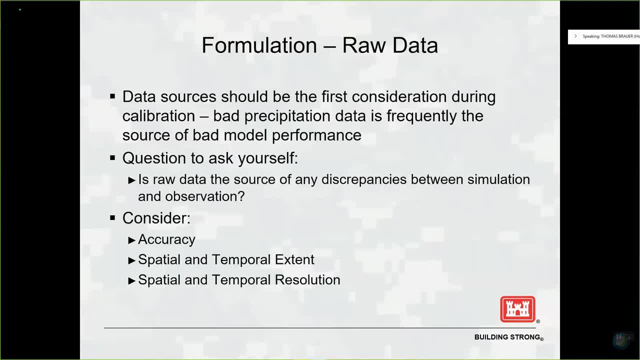 it during calibration. So yeah, if your model is bad, especially really bad, definitely recommend going back and reviewing your data. Boundary conditions actually are probably the highest amount of uncertainty out of anything in your model, And so things to consider is one: just take a look at the accuracy. 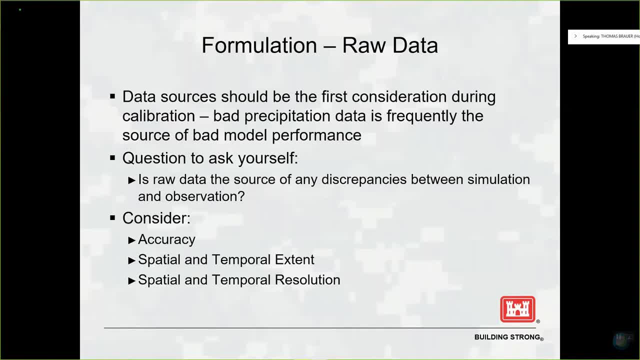 I mean, often I've tried to calibrate models and then once we go investigate one particular gauge, it's consistently bad And so that would be time to throw that gauge out. Other things to consider with the raw data: spatial and temporal extent. spatial and temporal. 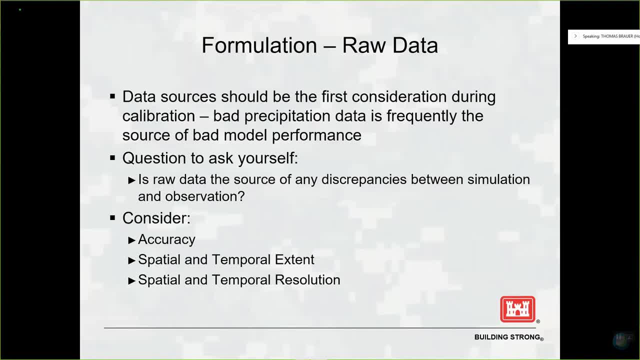 resolution. So what is like the time step of your boundary conditions And does it cover the extent that you're trying to model? And so things like: if you have a forecasting model, calibrating it with daily prism data probably isn't the best. 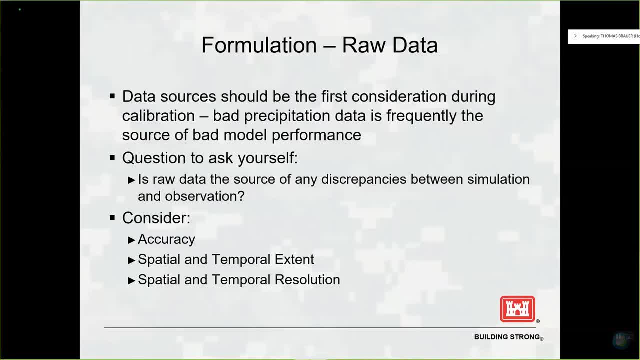 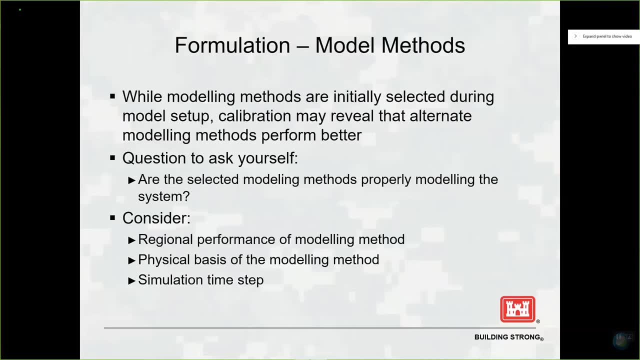 So you may want to make sure that the model is being calibrated to data that's going to be similar to what you're using in the forecasting context. All right, let's talk a little bit about modeling methods. So I mentioned event versus continuous earlier. 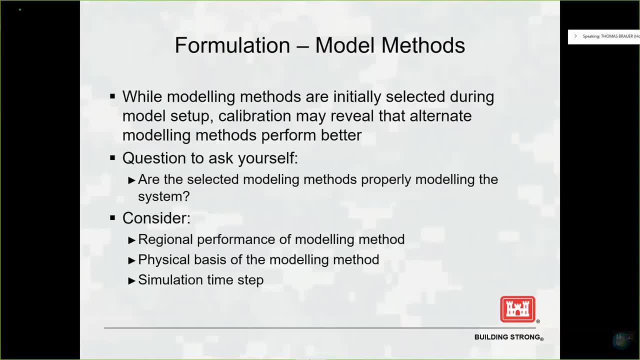 It's worth bringing up again on this slide. So modeling methods are just the methods included in a model, and one of the biggest ones we see come up again and again is event versus continuous. So I'm going to talk a little bit about that. 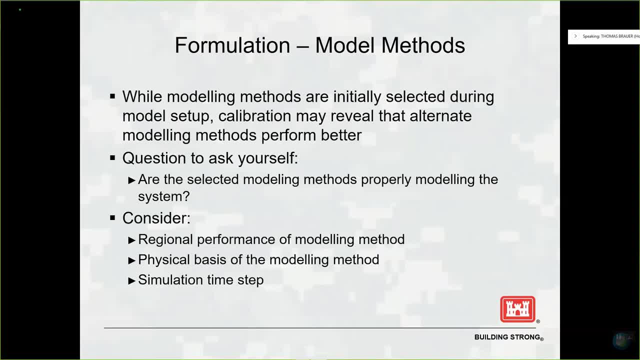 Event versus continuous. So often a model will be set up to do event modeling and somebody will try to apply it for continuous. The reality is continuous is not just a single event but often multiple events, And when you have a continuous model you have to consider more pieces of the hydrologic. 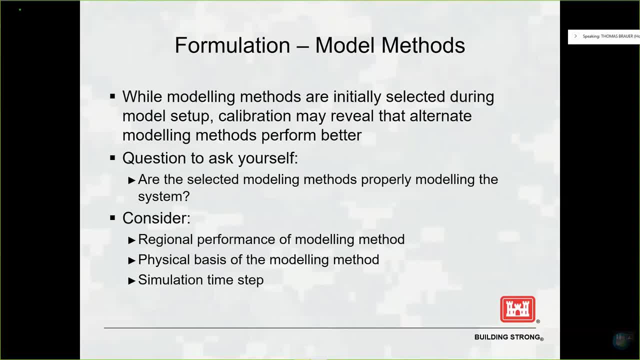 cycle. So precip on a basin isn't enough. We need to have evapotranspiration and soil moisture and base flow to truly capture a continuous simulation. So that's often this, you know. this formulation step is just looking at your model and how. 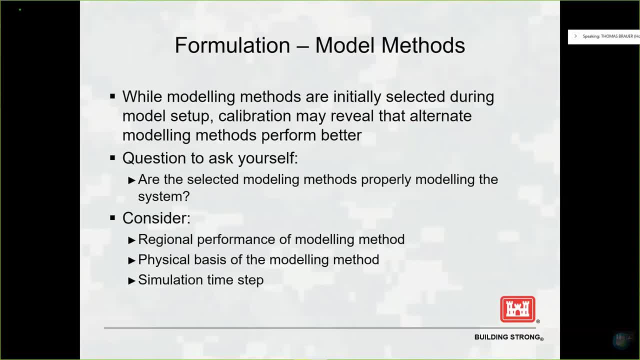 it's set up and is it capable to model what you're trying to do? So other things to consider, just the regional performance of the modeling method often, and then physical basis. So some districts have a history with a particular method and they know the parameters in their 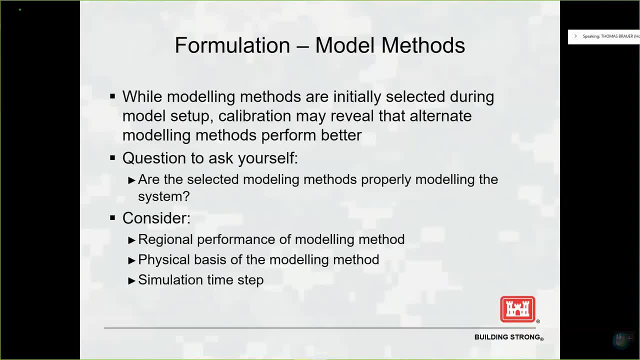 region. So if that's the case, it's probably a good method to use in your region. Okay So, especially if there's institutional knowledge, if you can go to a senior hydrologist at your district and say, hey, like, is this reasonable? 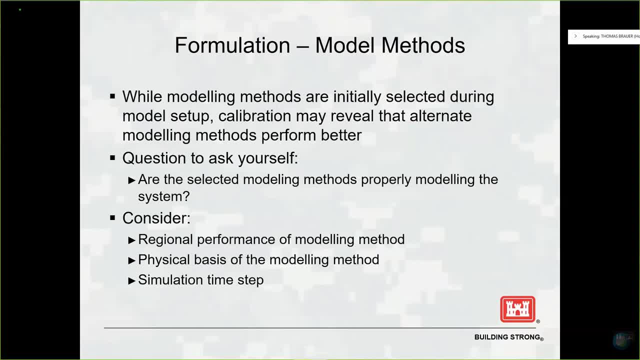 How should I adjust these parameters? That's usually valuable, So definitely a consideration. And then physical basis, so just with physical methods. often the parameters are kind of tied to physical measurements, or they're supposed to be, So things to consider there. 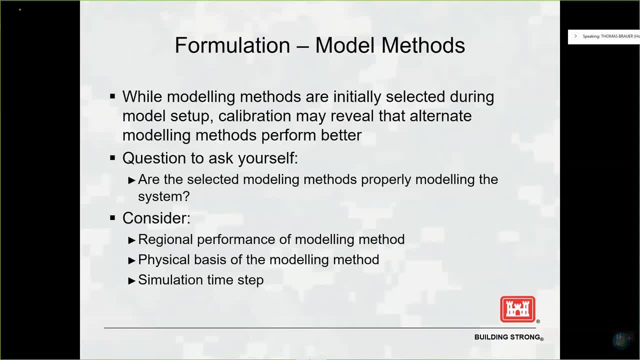 Is this physically based? How adjustable is it? Or is it empirical? Is this coefficient? Can it kind of widely range? So let's talk a bit about parameter adjustment. This is a step most people think of in calibration. So this is when you have your model data. 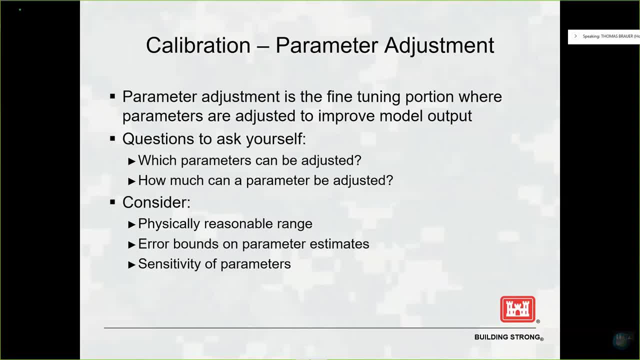 You're taking a look at it, It's good to go And your methods are where you want them. This is often the place you'll find yourself in in the forecasting context, because a lot of these models have already been built And there's been years of history and tradition that have, you know, led to the decisions. 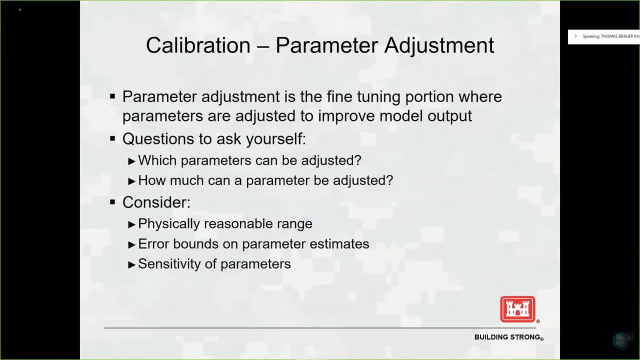 that were made to set this up. Like we know, this is going to do the best transform method. We know that gridded precip is the best for forecasting, So you're probably going to find yourself in this spot in the forecasting context. 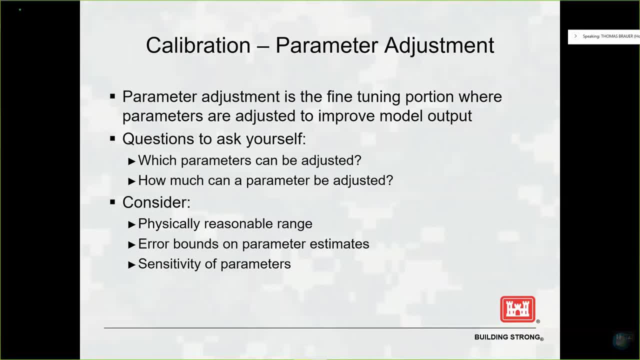 And so parameter adjustment is just the fine-tuning portion where we adjust the parameters to improve model output. And it's a question to ask yourself which parameters can be adjusted and how much should they be adjusted. These are very important questions. 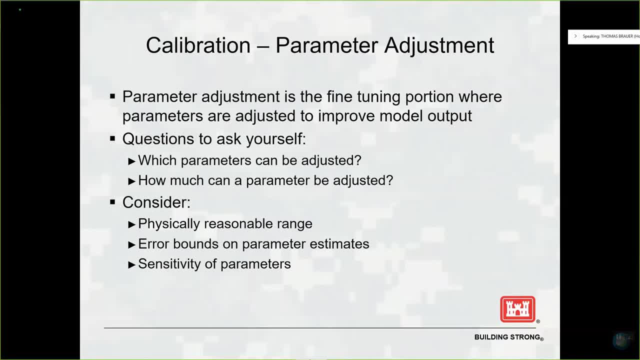 Obviously, parameters that are really physically tied can be adjusted a whole lot And, for lack of a better example, things like a reach length, like- okay, like people actually do change that from time to time, But it's very physically-based. 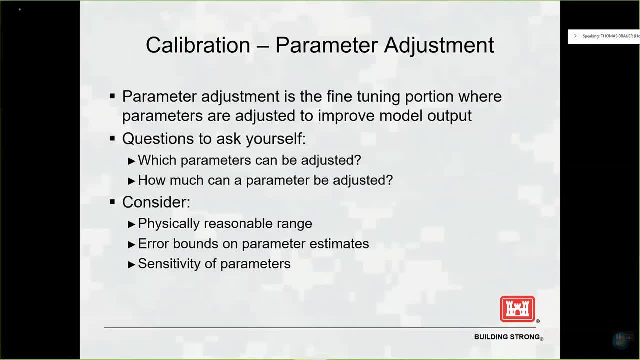 So there's not a whole lot of adjusting that can be done there. Other parameters, like TCNR, you know for your transform, those have a pretty big range of adjustment, But then again there's a limit to that And so it's just really you as the modeler need to get a feel. 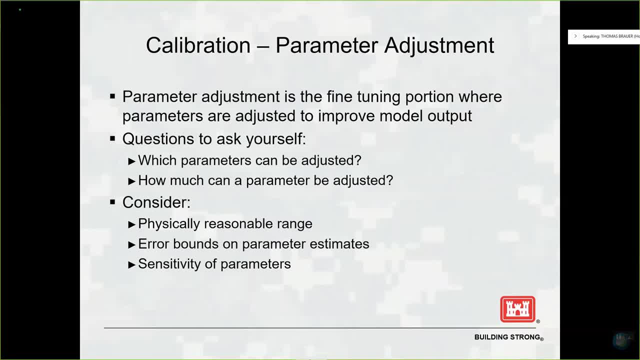 Especially in your region, like what should these parameters be and what's a good range on them? And so one of the best ways to get a feel is to do some modeling and train your data on training data sets. So run it for events that are similar to the types of events that you'll encounter. 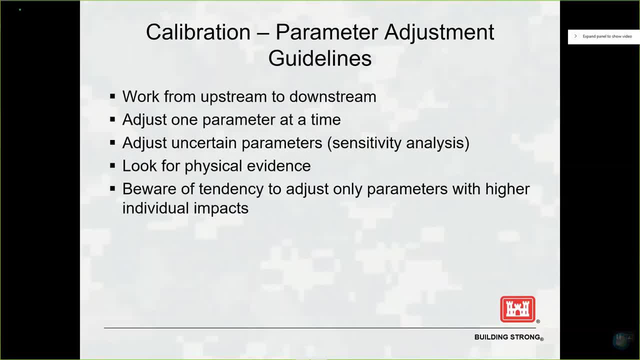 in forecasting. So here's some guidance on calibration. You want to work from upstream to downstream. You want to make sure that your headwater sub-basins are calibrating, because there's no sense in trying to calibrate something downstream if the upstream is not calibrated. 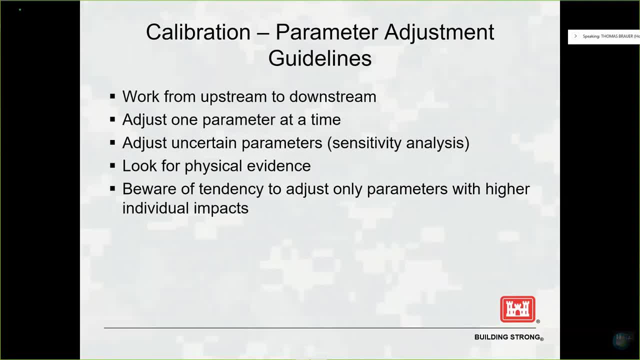 Okay, That's pretty intuitive- And then adjust one parameter at a time. This helps you isolate and get really good control on your experiments, Because you're just kind of making adjustments, experimenting- okay, is this doing what I want to? And so when you change multiple parameters at one time, it's easy to get confused, as 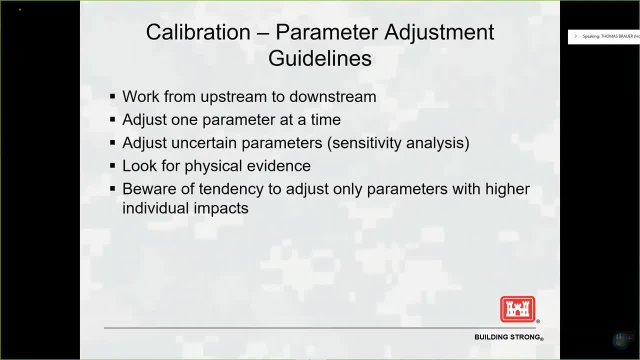 to what's causing what And then adjust on certain parameters. So things that have a range, like TCNR, like you want to start focusing on those, Adjusting those, Do a bit of sensitivity analysis and seeing how much does this change the result. 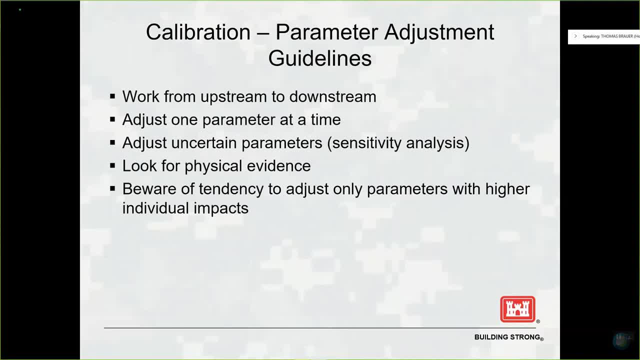 Look for physical evidence, So something like a loss method. You want to you know. so if you increase your constant rate, so you increase the rate at which water percolates through the soil, is it bringing down the peak? So you want to see that what you intuit by changing the parameters is actually happening. 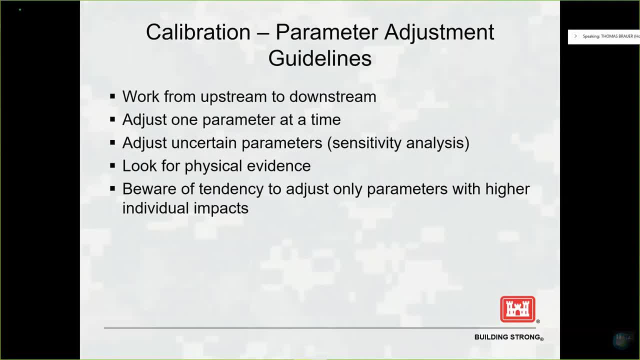 in the model And then be aware of tendency to adjust. It's only parameters with higher individual impacts. So this is what's called in the model world overfitting. So if you see, oh, okay, like if I start adjusting this base flow coefficient and I 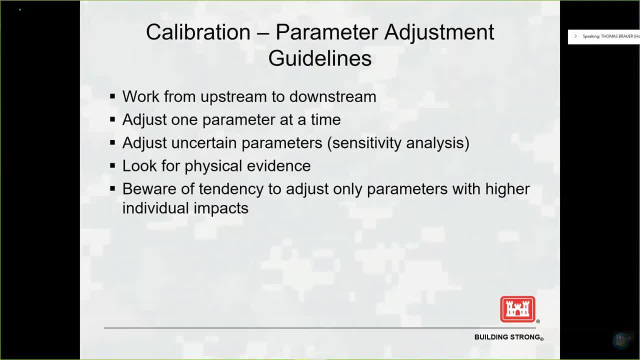 really crank it up. I'm getting a better result in this model, even though it seems like you know, it might be out of range or it's a little bit too much, but it gives me a good result. The reality is that when you do that, if you try to apply that model to say a different, 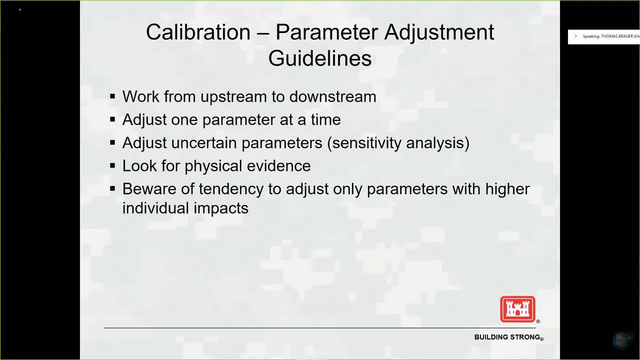 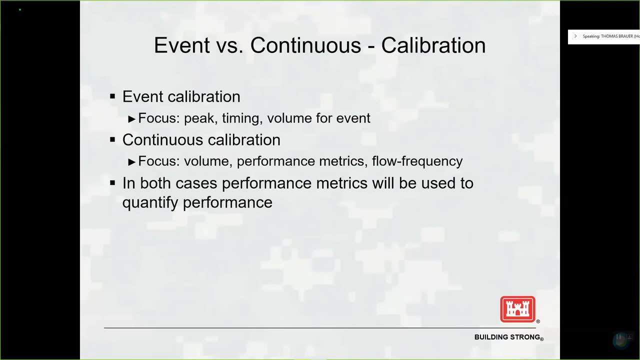 event. It's very likely now that that next event is going to be, you know, very wrong, So it's important to not overfit them all. Okay, So I distinguished event and continuous a little bit earlier. Once again, event is it's something on the order of days? 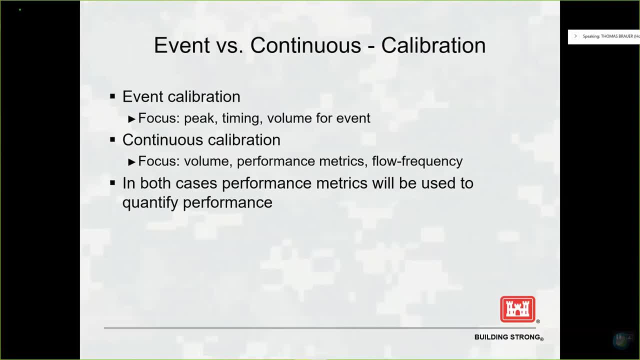 Maybe a week, So like seven to ten days at most. The point at which other hydrologic processes start to come into play, Things like base flow and evapotranspiration, Like if you're modeling long enough for those processes to come into play, then that gets. 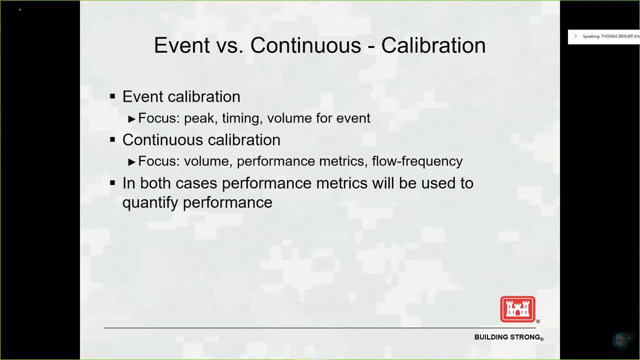 into continuous calibration, And that's when you need to start modeling those processes in your model. And so, with event calibrations, these are usually focusing on the peak. What is the peak amount? Emily's going to show these The timing. 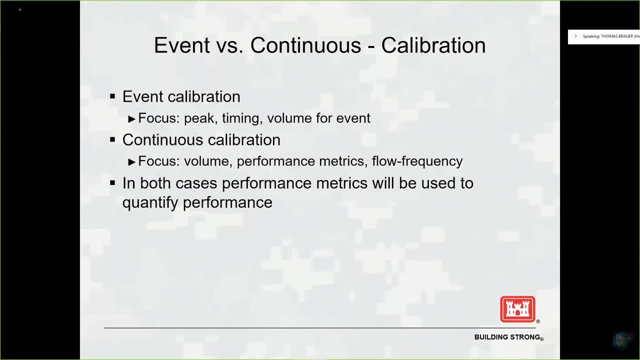 Like what is the timing of the peak And then the volume for the event. So with continuous calibration, the focus is often on volume And then we use performance metrics. It's often hard to view the entire because with event calibrations we're doing this. 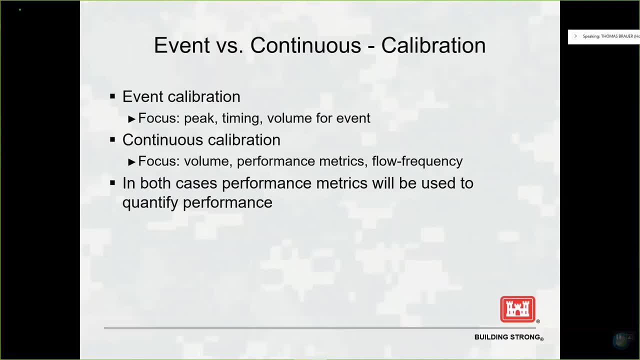 often doing a graphical inspection where we just look at the hydrograph and we look at the fit. With continuous calibration it becomes more difficult to do that type of inspection. So that's where performance metrics really help us there. And then for really long continuous calibrations we might start looking at flow frequency. 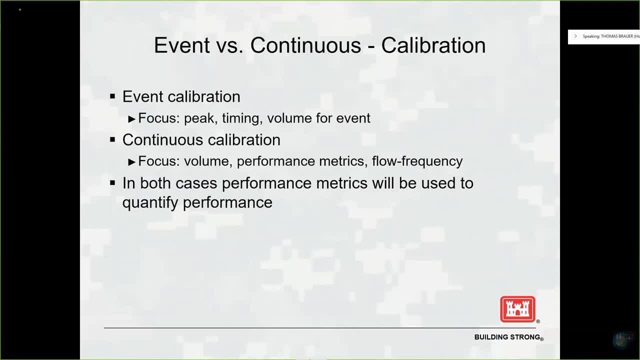 We might start looking at flow frequency curves and seeing if we can reduce the flow frequency curves or reproduce the flow frequency. So it's really just a matter of getting things into a view that we can process like a flow frequency curve. We can't look at the fit for the entire 60-year simulation of a continuous model, but we can. 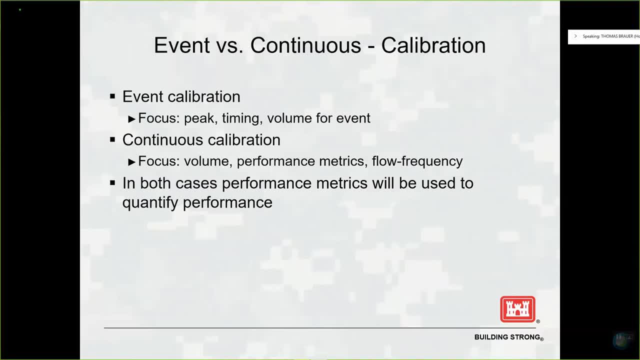 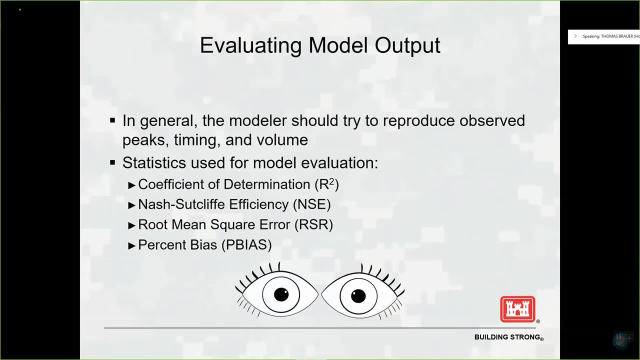 look at a flow frequency curve, can look at performance metrics. And then the last little point here: in both cases performance metrics will be used to quantify performance. So graphical inspections are great, but performance metrics are kind of a common way to communicate. 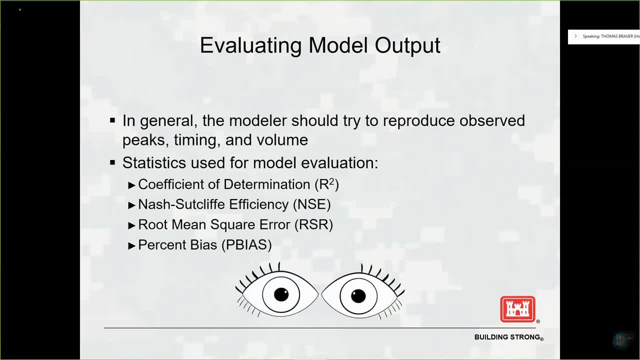 model performance. So you can. you know, one person can look at a curve and say I think it's good, And then the next person says no, that's not a great calibration. So there's some subjectivity there. 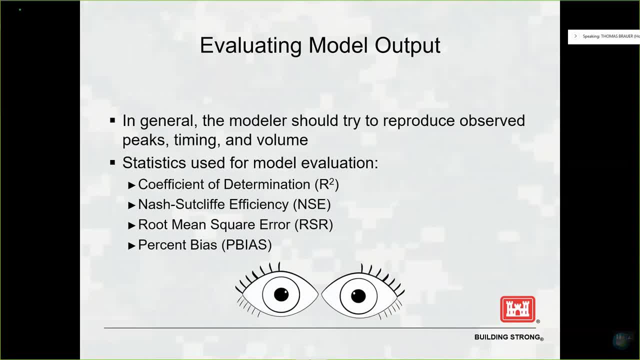 The thing that we get with these statistics is a common measuring stick for how the model performs. So we tend to use these statistics in both continuous and event, and any time you're putting together a report, it often you know you'll have a list of these statistics and 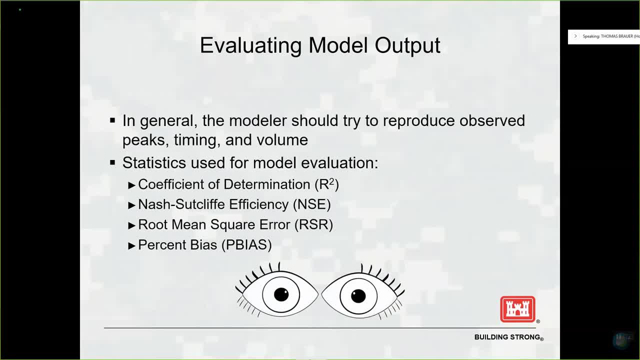 how each calibration location performs, So statistics that I guess all of these are usually used in the reports. There's two that we often look at and I think most of the modeling community, at least the UCS community, looks at while doing calibration. 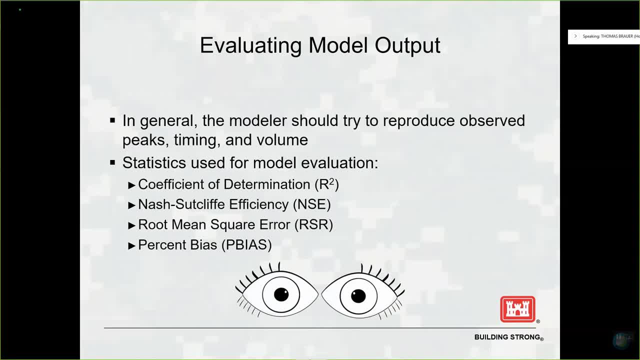 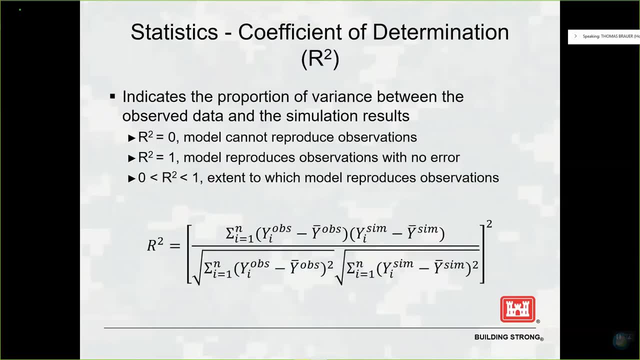 Those are the nashcliff efficiencies, So we'll go ahead and mention the others, because you'll probably be doing a report at some point where you'll want to include them. So the coefficient of determination R squared. you probably remember this from a college-level. 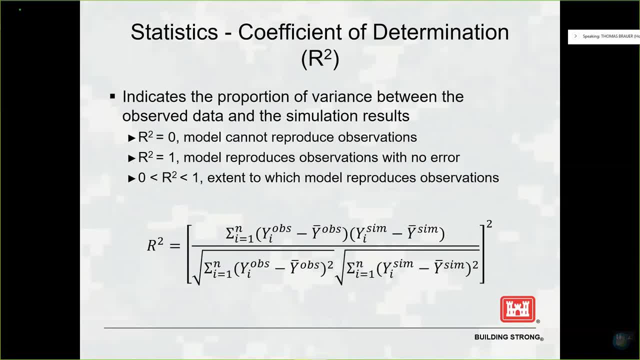 stats course. Let me just refresh you. So an R squared of zero is that the model can't produce observations. An R squared of one reproduces observations with no error, And then somewhere in between is the extent to which the model would produce observations. 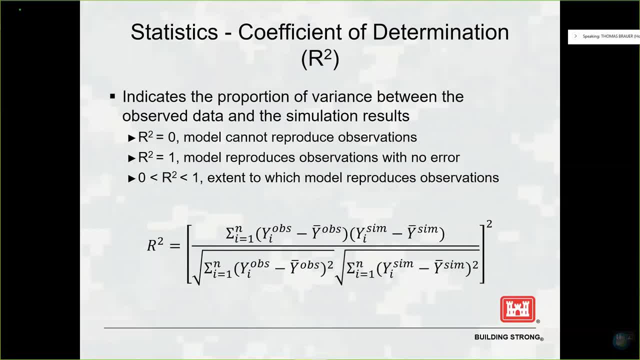 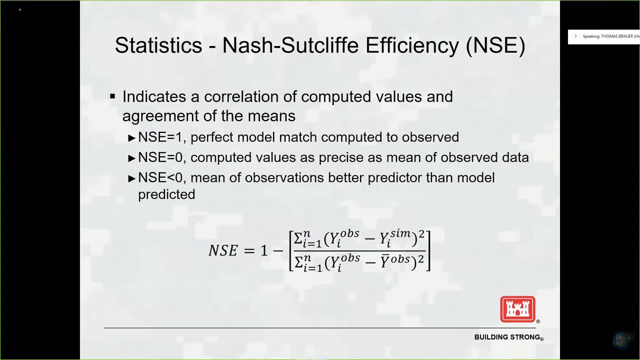 So I have a slide here and a couple of slides where we'll show reasonable or we'll qualify the metrics. So what's a reasonable or good range for these statistics? The nashcliff efficiency indicates a correlation of computed values and agreement of the means. 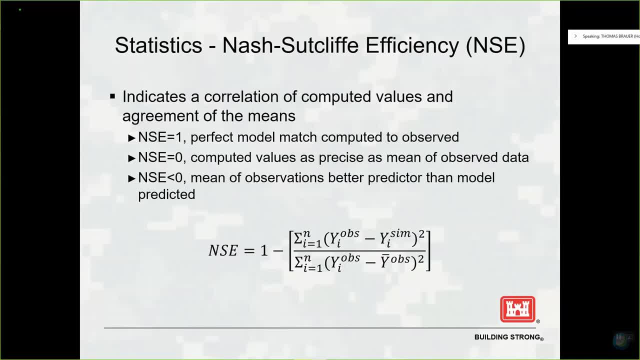 So this is really just the fit. This is the metric for how well the curves fit. the simulated versus observed Nashcliff efficiency of one is a perfect match between computed, observed and observed. Nashcliff efficiency of zero is that the computed values are as precise as the mean. 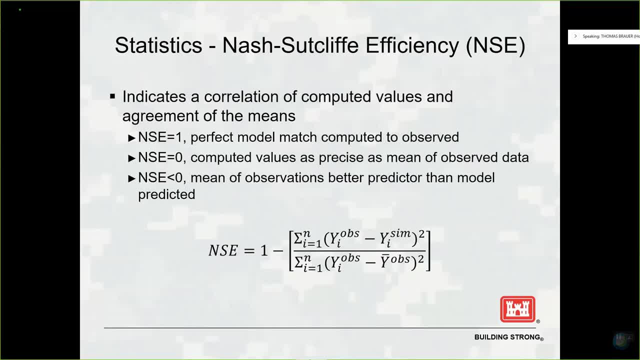 of observed data, So that's really getting into pretty bad territory. Your model is not as good as just taking the mean of all of the observed data and projecting that forward, And then less than zero is getting really bad. So the mean is a better predictor. 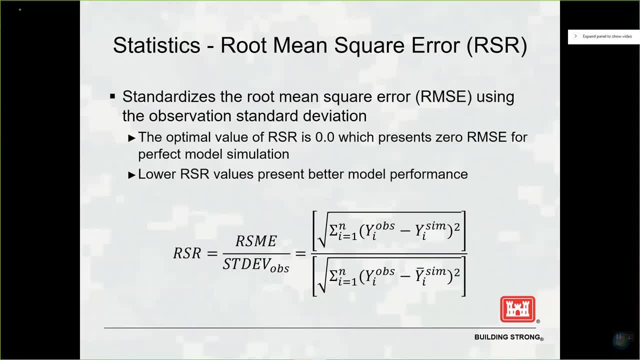 And the model predicted: Root Mean Squared Error Standard Deviation Ratio. So the metrics. these metrics all came from a paper, and this is one of. it's called Mori et al 2007.. There's a reference here in a couple of slides. 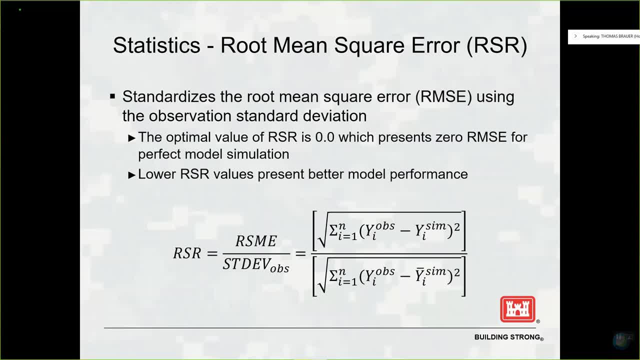 And so this is one kind of a new statistic they proposed, And so we often use it in our reports. The optimal value is zero, which means zero root, mean squared error for the perfect model simulation, And then lower RSR values represent better model simulation. 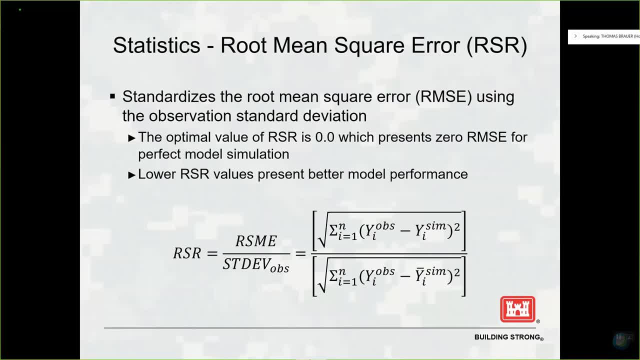 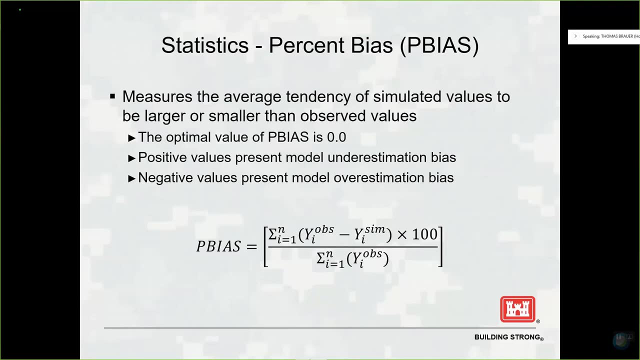 So this one, the first two, I showed you coefficient determination and the Nashcliff efficiency. the perfect good value is one. For RSR, the perfect value is zero. And then let's take a look at percent bias, And we use percent bias to give a notion of volumes. 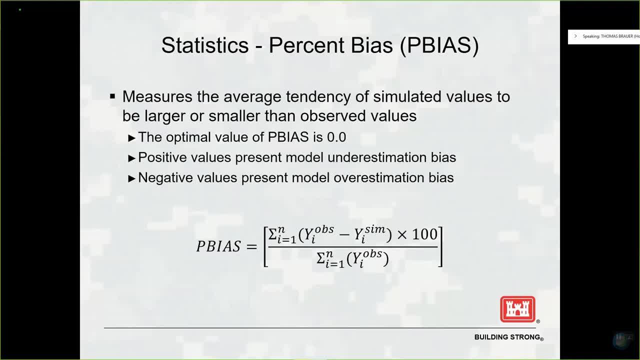 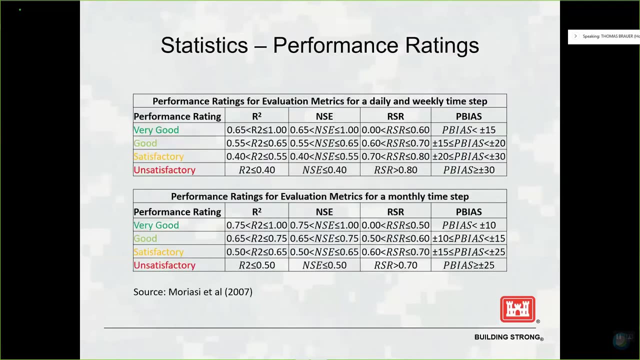 And so this measures the average intensity of simulated values to be larger or smaller than observed values. The optimal value is zero, And then negative. positive indicates overestimation or underestimation. So is the volume greater than or the volume less than? 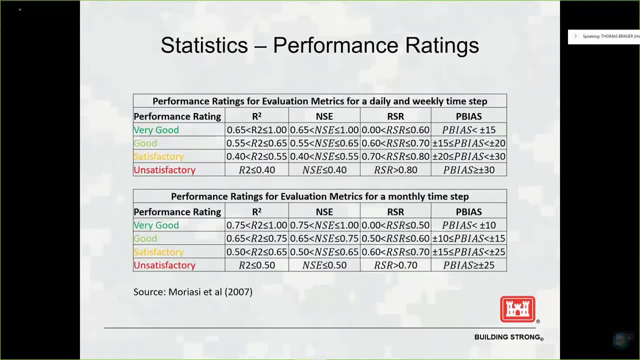 And then here's that table I was talking about. So, with each of these statistics, this Mori et al paper 2007 publishes ranges as qualifying each of the statistics in a way: So very good, good, satisfactory, unsatisfactory. 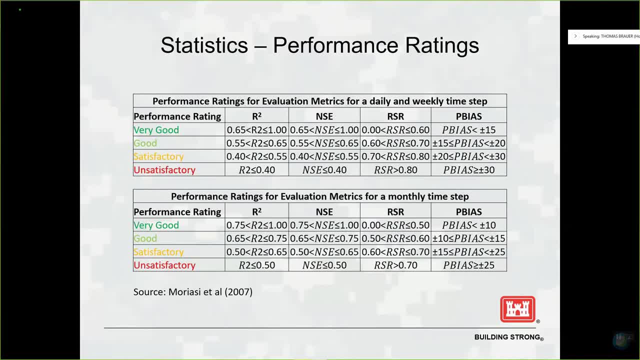 I think this has been passed around a lot, So if you haven't seen it before, you've seen it now and you have these slides, And so hopefully you can use this as a guide when taking a look at your model and how it. 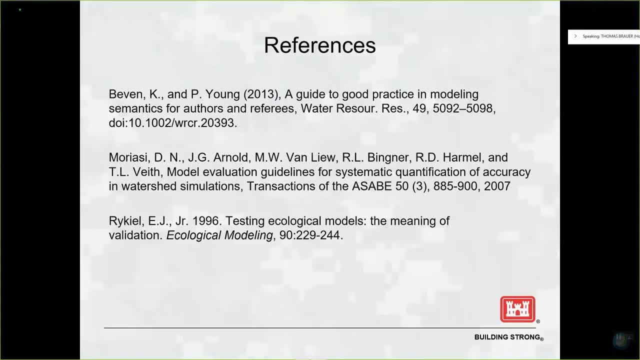 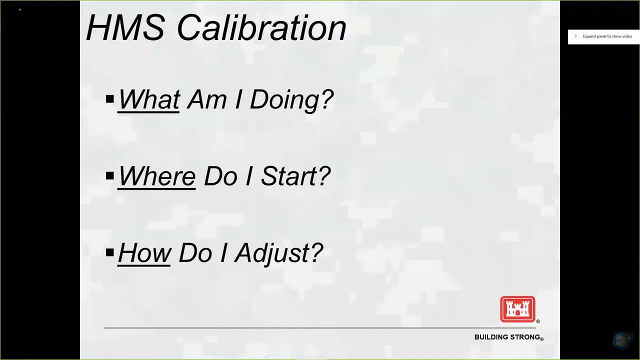 calibrates. So there's those references I mentioned. in case you want to go take a look. And now I'm going to pass to Emily. All right, I can't hear Emily now. Well, thanks, Tom. And, as Ann mentioned, I'm Emily Moe and I'm from the St Paul District. 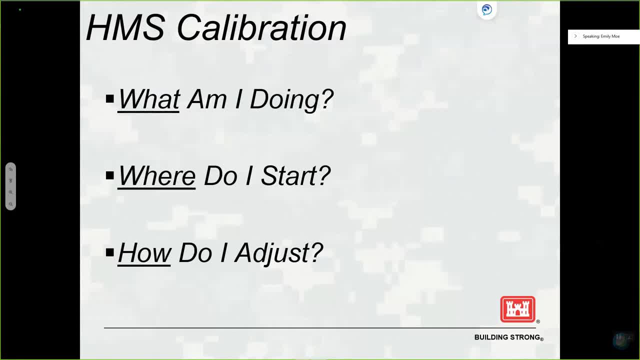 And I have a lot of experience developing our HMS models, And so what I'm going to share today is kind of some tips and tricks when you're learning HMS, because I've helped a lot of folks kind of get more familiar and learn how to calibrate. 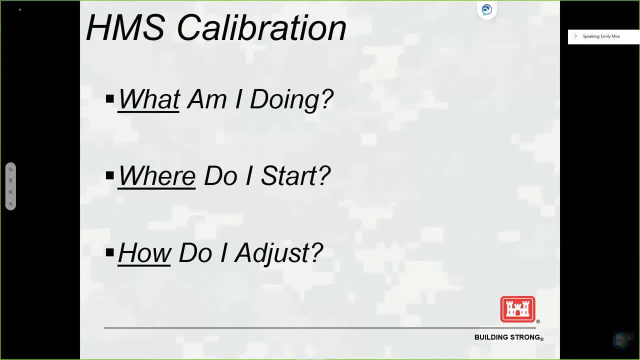 And it seems like it's a pretty good approach if you kind of break it down into three questions. when you're learning HMS One, what am I doing? and then, where do I start and how do I adjust or calibrate these parameters? 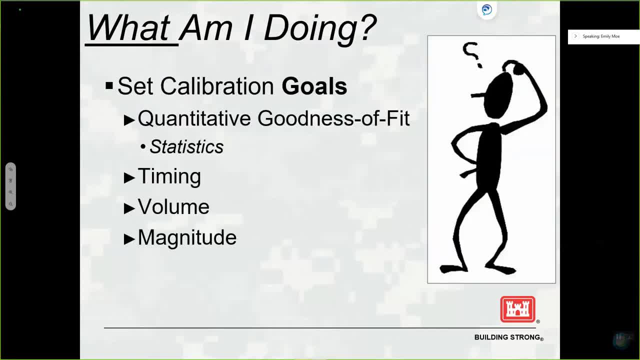 So, first of all, what the heck am I doing? It's really helpful when you're preparing to calibrate a model, to set goals. Some of the calibration goals you might set would include a quantitative goodness of fit, using some of those statistics that Tom talked about. 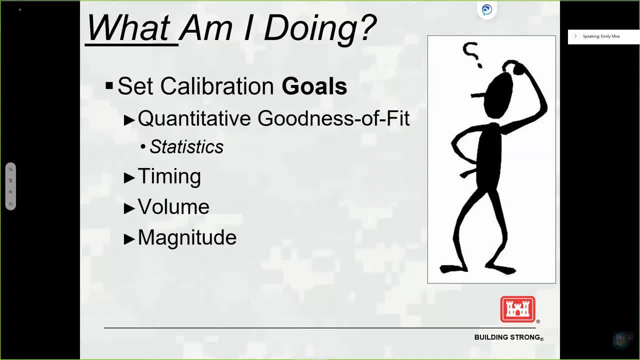 Other goals would include how important it is to your model and the objective of your project to capture the timing, the volume and the magnitude of the calibration event, And we've got some examples of goals included in the next few slides, but these goals can 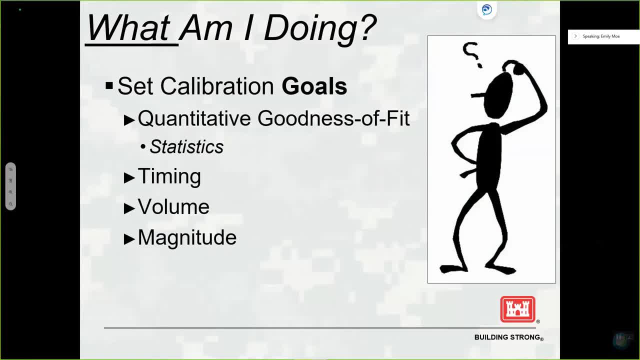 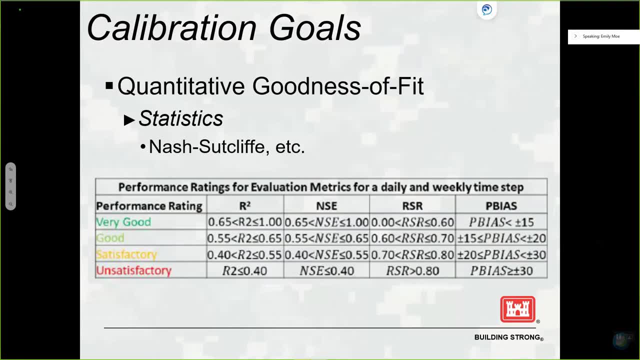 definitely vary depending on the purpose of your project. So, first of all, it's great to set some quantitative goals using statistics instead of simply making them out using the eyeball test, because, like Tom mentioned, what looks good to one person might not look as good to another. 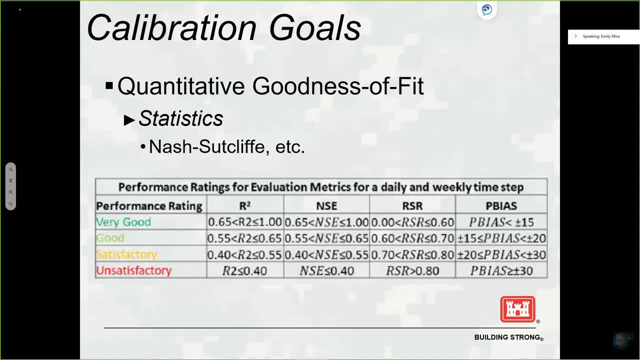 So by leaning on these statistics and setting goals such as the R-squared or the Nash-Shutcliffe- which is what we kind of rely on the most in the St Paul district- it's a lot more clean cut as to whether or not this is an acceptable calibration or not. 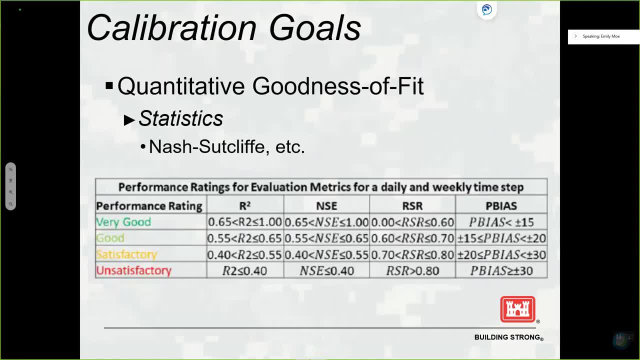 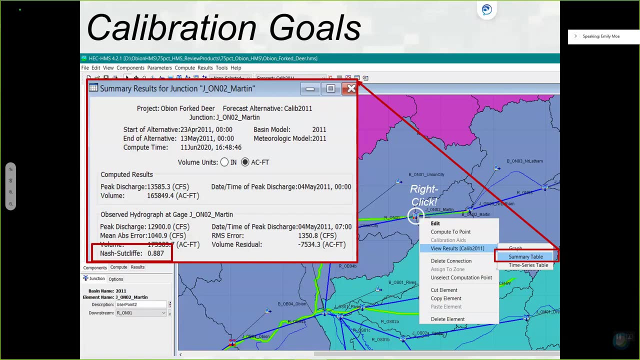 So, for example, to be considered satisfactory from this table, the Nash-Shutcliffe coefficient should be greater than 1. And if it's above 0.65, it's considered a very good fit. So, thankfully, if you have observed flow data linked to a junction within HMS- HMS itself- 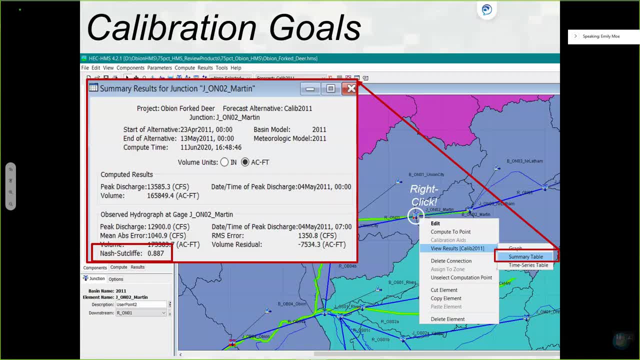 will actually compute several goodness-of-fit statistics for you, And these statistics can be found in the junction summary table by right-clicking on the junction and selecting View Results and then Summary Table. So, for example, here you can see that there's the Nash-Shutcliffe coefficient. 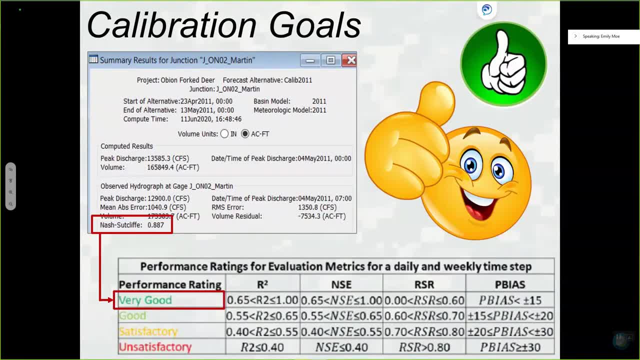 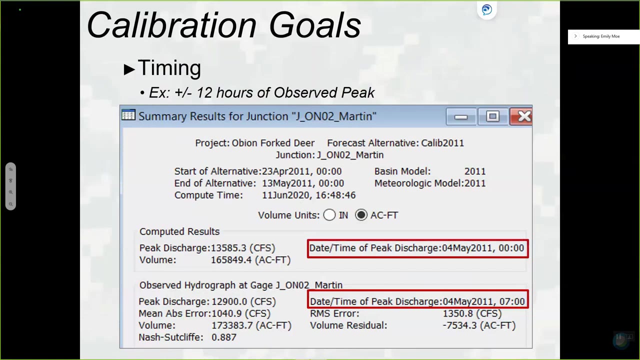 And this particular location and event has a Nash-Shutcliffe value of 0.887, which we saw into the Very Good category. So technically this is a statistically good calibration here. So beyond simple statistics, it's also really useful to set calibration goals for other. 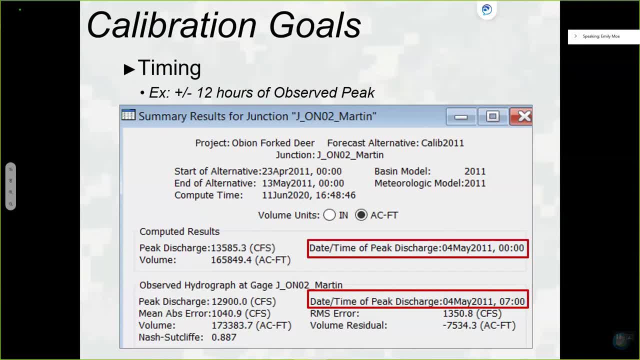 event components that are based on the objectives and needs of your project. So, for example, up here we have the Nash-Shutcliffe value of 0.887.. So for example, up here in St Paul for our SWMS, HMS models, we've kind of set an initial. 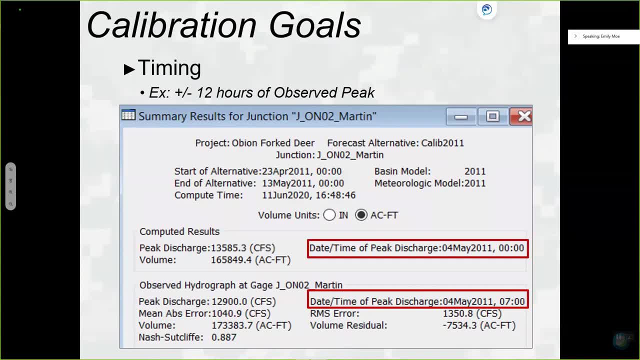 goal of calibrating the timing of events to within 12 hours of the observed peak. Again, the timing goals can vary significantly based on what the objectives of your project are. So if you're not doing a SWMS model and you need things to be more exact, they might be. 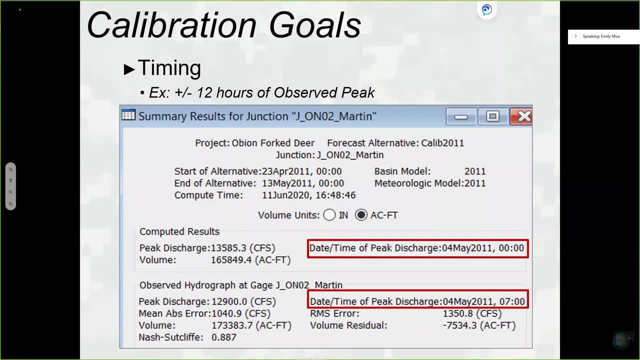 a little more refined, But HMS makes it really easy to compare the modeled and observed peak timing by displaying both timestamps within that summary table. So if you're not doing a SWMS model and you need things to be more exact, they might be a little more refined. 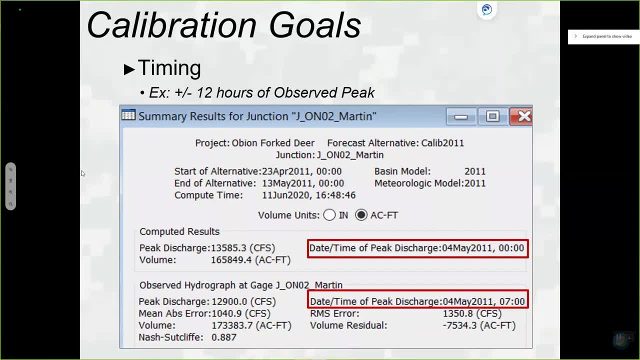 The timing goals are listed here in the SnT gedaan ducts window, as shown here as well. All right, so volume is another key component of each calibration that you should take into consideration when you're setting your goals, Particularly if you'll be using the HMS model for SWMS or for other reservoir studies. the 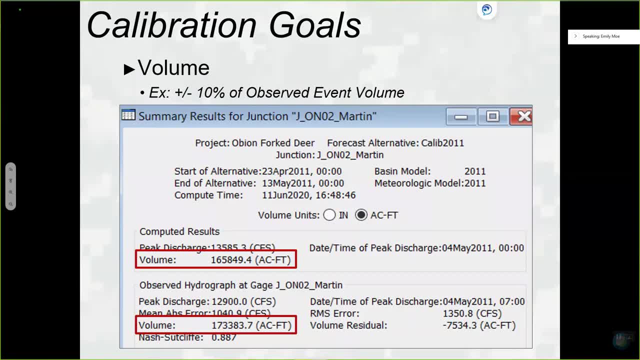 event volume is a critical component that you'll want to capture as closely as possible. And up here in St Paul for our SWMS models, we set an initial goal of capturing the complete �를p Wiseman, capturing that total event volume within 10 of the observed event volume. and again, hms makes it. 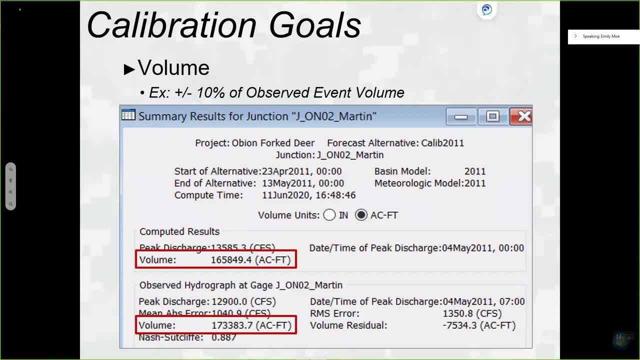 really easy to obtain the models and serve volumes through the event from directly within the summary table at each junction with the third data. so event magnitude is another component that you might consider setting calibration goals for often the peak magnitude corresponds to the peak stage and innovation levels. so depending on the scope of your study, the magnitude goal may vary up here. 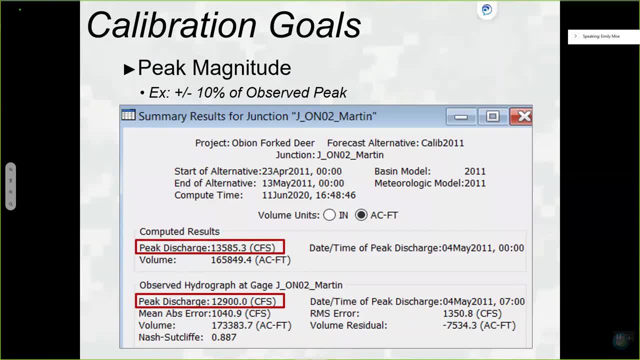 in st paul for experience models we set an initial calibration goal of coming within 10 percent of the observed peak magnitude um and again looking at the summary table hms makes it really easy to do a quick peak magnitude comparison between the modeled results and the observed values. if you 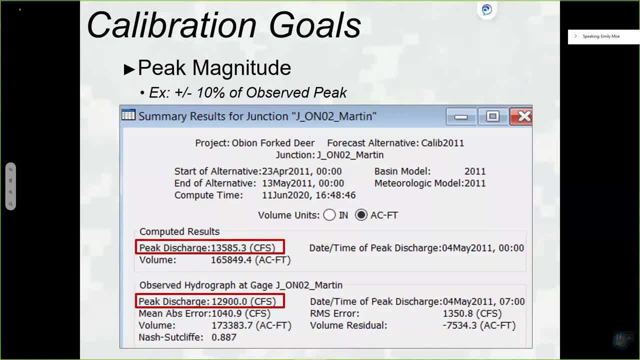 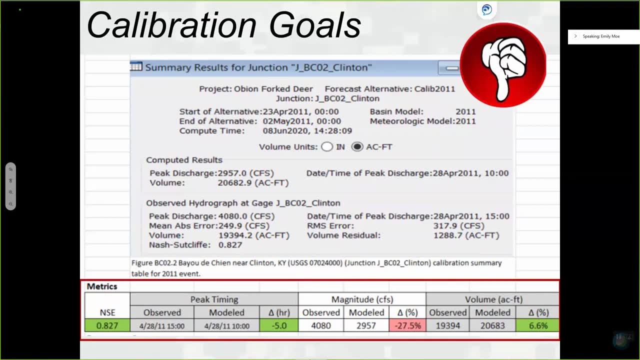 have have that data linked to the junction uh. so the hms junction summary table provides a lot of really great information that's available really quickly after you run your your model. however, it won't compute the percent differences or alert you as to whether or not you're meeting your calibration goals that you set. so one thing that i found: 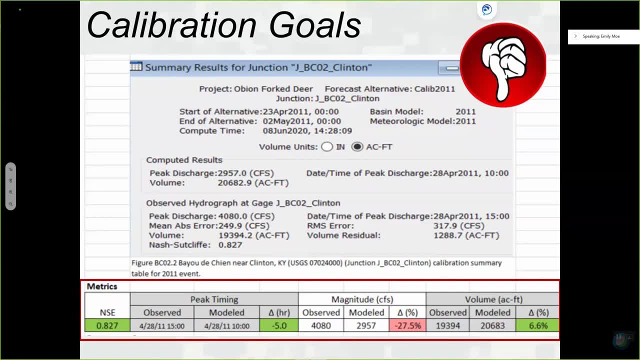 helpful is to use a spreadsheet that's set up to manually answering your results. but then the spreadsheet is programmed to compute the timing or the percent differences and it's color coded to show green if you're within the range of your goals or red if there's still work to do, like the magnitude shown in this example. 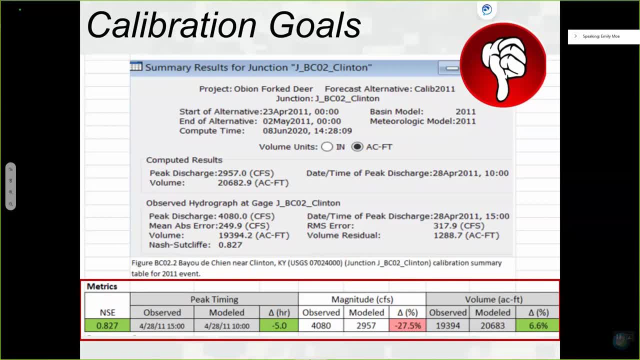 but after, uh, so we can quickly just pop that into the spreadsheet and see up, we've got a, we've got got some reds. we've got a little bit more work to do and if we adjust it a little bit more, we've brought it back into within the range of our magnitude goals there and we're meeting the 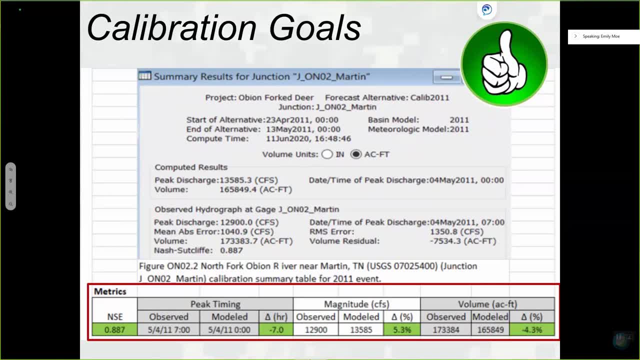 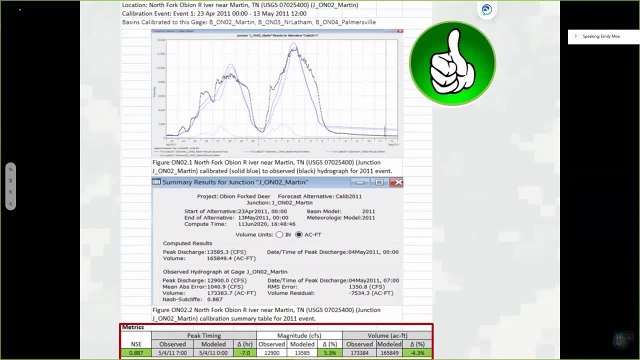 rest of our goals, so everything's all green and looking good, and i found that kind of developing a tool such as this. especially if you have a large watershed where you're- you're looking at these percent differences and timing comparisons for several, several locations- it's really nice to kind of have this ready where you can just type it in and instantly know. 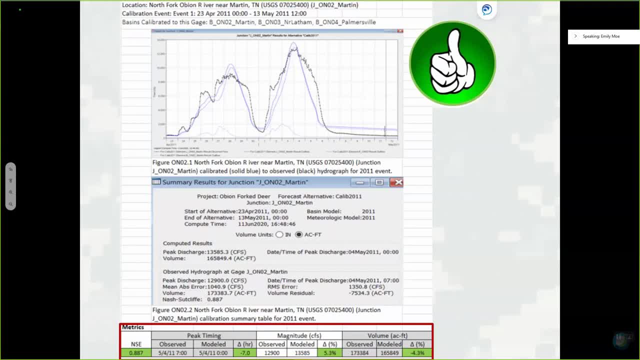 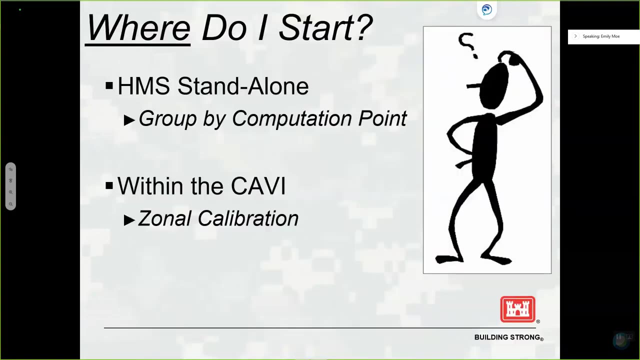 instead of having your hand computer over and over again. and it's also really useful for documentation and for reporting purposes as well by providing a consistent template with all of the key information from the calibration present in in a glance there. um so, once these calibration goals have been set, where does the modeler start the calibration? 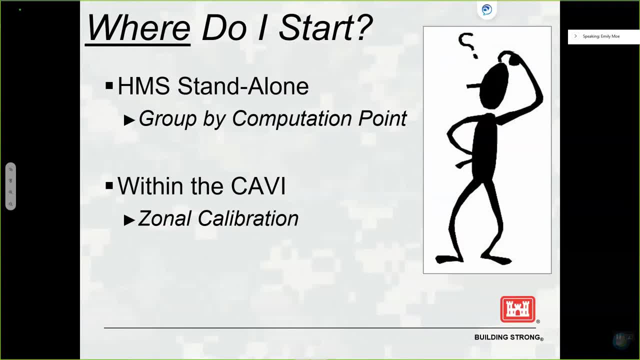 process, and for this there are really two main options when using hms. one, you can use hms standalone or- and by standalone i mean you're launching the software program outside of this lens caddy for calibration purposes, or you can actually launch and use hms directly within the. 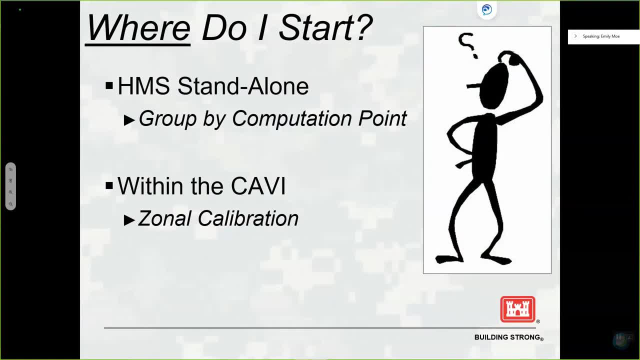 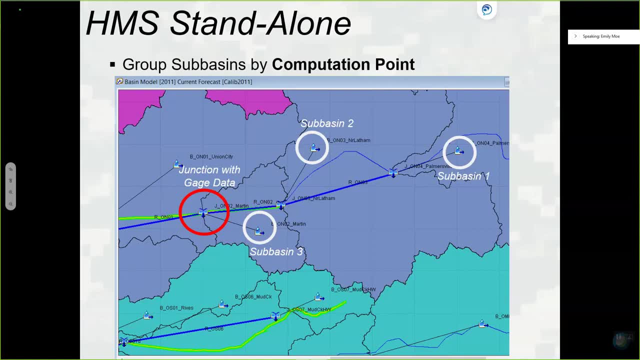 caddy too, using zonal calibration, which may be more common for a daily slim forecasting effort. so when you're using um hms standalone or opening it outside the caddy, when you're calibrating it's really useful to group sub-basins and to calibrate by computation point. so, as tom mentioned, 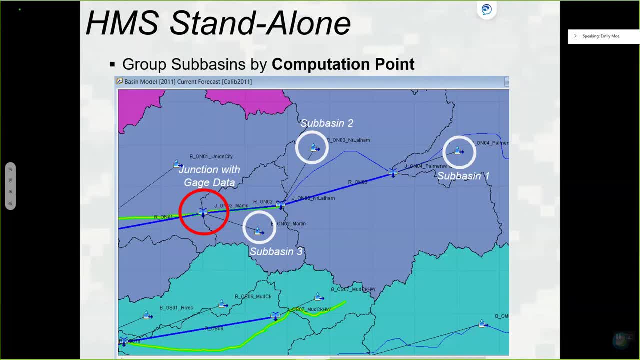 it's good to start at the headwaters or your watershed. so here's an example up in the headwaters, where there are three sub-basins that are above a gauge location and it's helpful to group these sub-basins by flagging that gage location and it's helpful to group these sub-basins by flagging that. 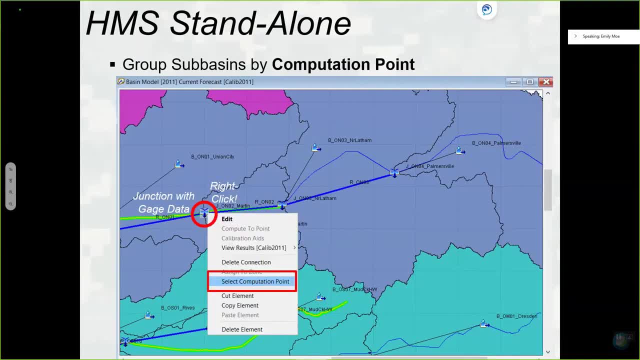 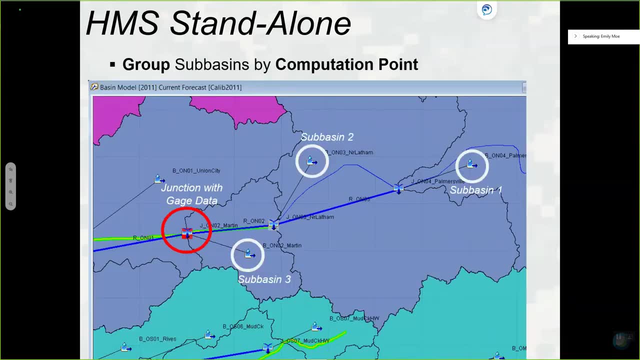 gage junction as a computation point, and to do this you can simply just right click on the junction and select computation point, and this then turns the junction icon to a red shade, which denotes that it's been marked as a computation point. and flagging this junction as a computation point then groups these sub-basins that are: 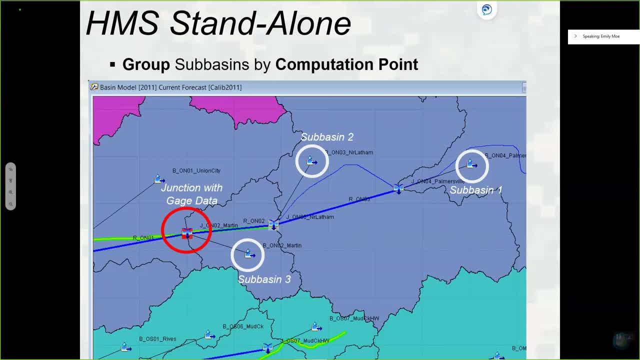 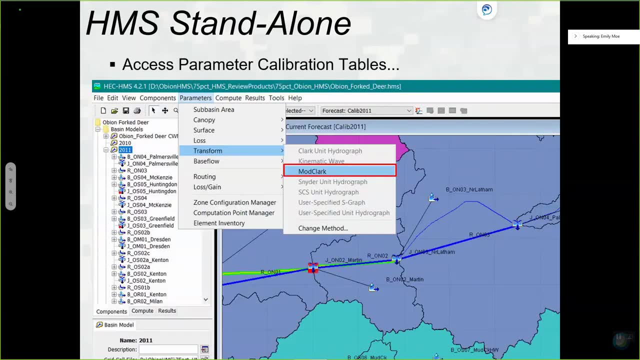 located upstream of the junction together into into a group that's associated with this point. so now, now you flagged this group, you can access the parameter tables by by the method, and right here we're going to look at the transform method, which in this instance, is mod clark. 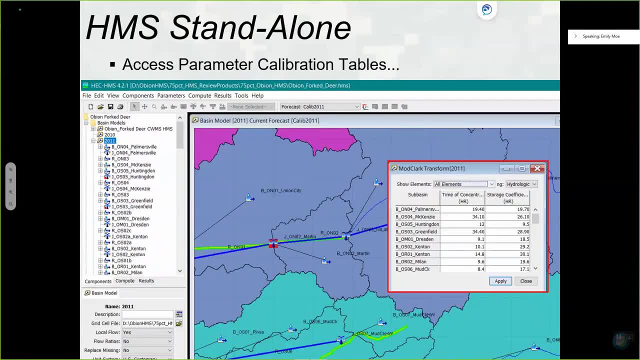 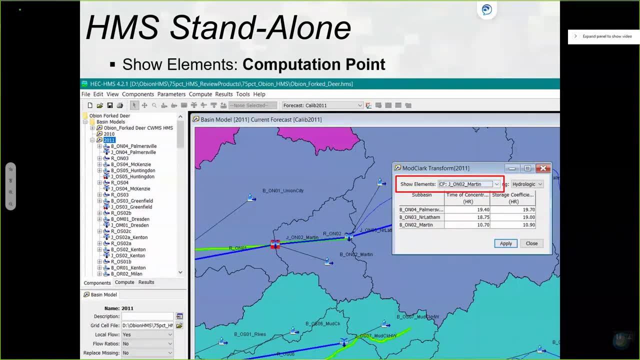 and by selecting this it launches a table dialog with all of the sub-basins and their associated transform values listed and from here the sub-basins can then be filtered through the show elements option by selecting the computation points that we just flagged from the drop down menu and filtering that computation. 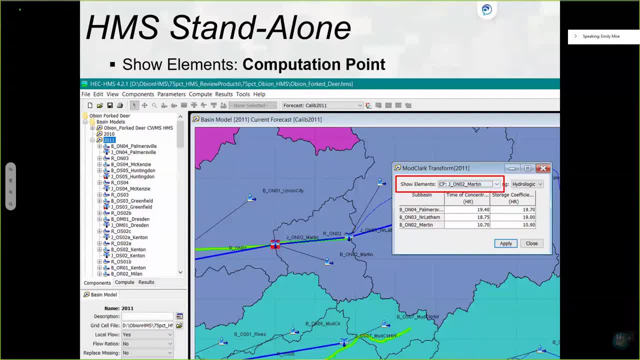 point then displays only those sub-basins that have been grouped to that point. so in this case, it's the three that we were just looking at, and what we see here are the initial values that were estimated based on some sort of analysis, whether it was gis or previous model values or whatnot. 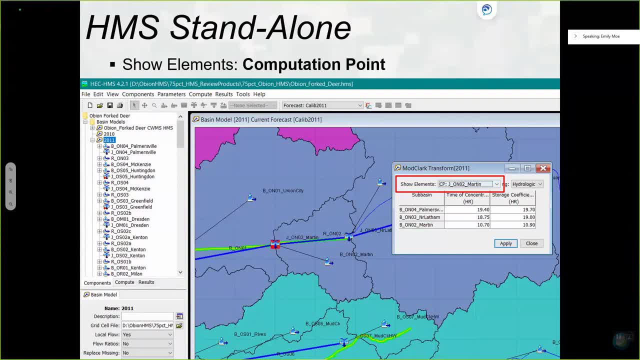 however, these initial values are really just an educated best guess of what these values may be before calibration. so a good next step in this practice is to adjust these parameters by group instead of adjusting each sub-basin individually. adjusting by group allows the sub-basins to 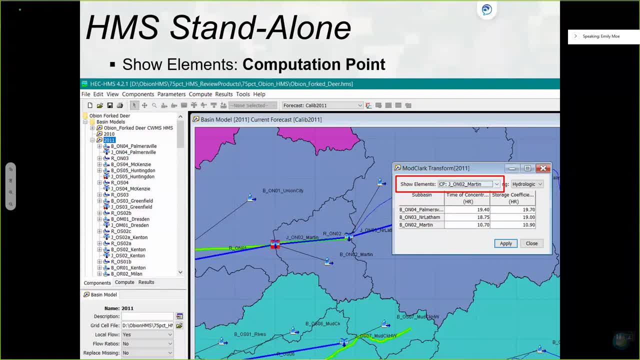 maintain the scalar differences that were derived from those initially estimated values. so, for example, if sub-basin a was twice as large as sub-basin b and the initial estimate of sub-basin a travel time was about twice that of sub-basin b, if we scale the travel travel time values, the tc values, by: 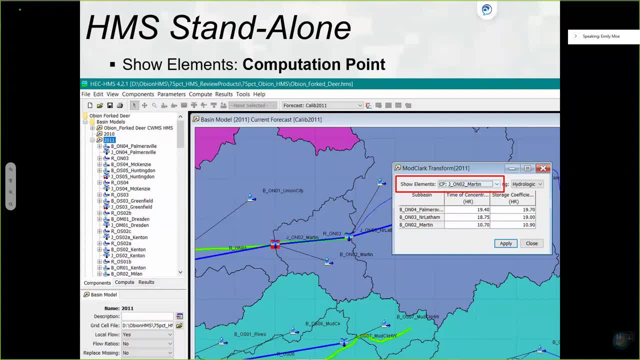 group, then the final tc value for the larger sub-basin will still be about twice that of sub-basin c, the smaller one, and we'll simply have scaled those initial values to best match the observed data. we still maintain the approximate differences between those sub-basins. 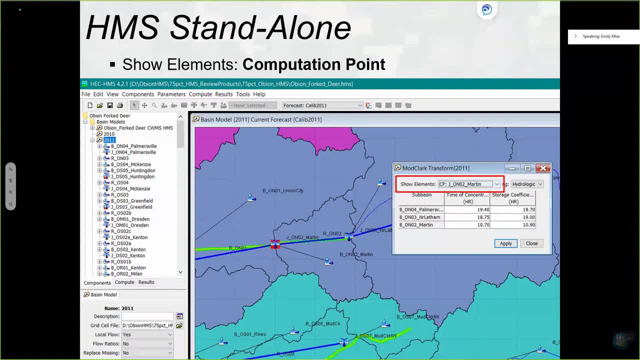 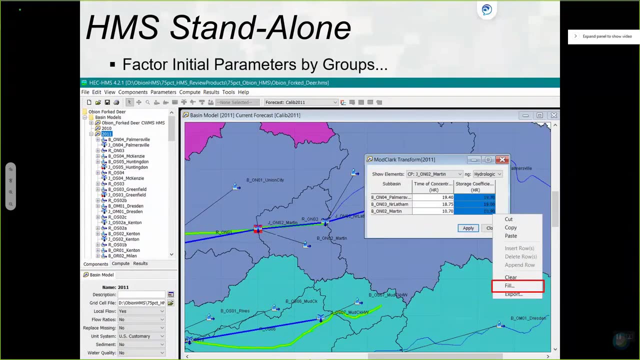 that were originally developed. so this approach often works really well when there are several sub-basins that are upstream of a single gauge and there's really no intermediate observed data to justify adjusting them individually. so in order to scale these values as a group, you can simply 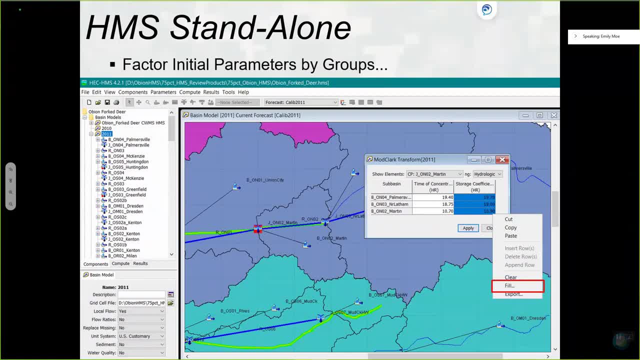 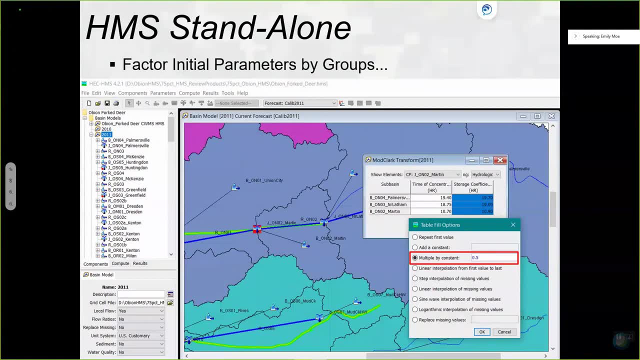 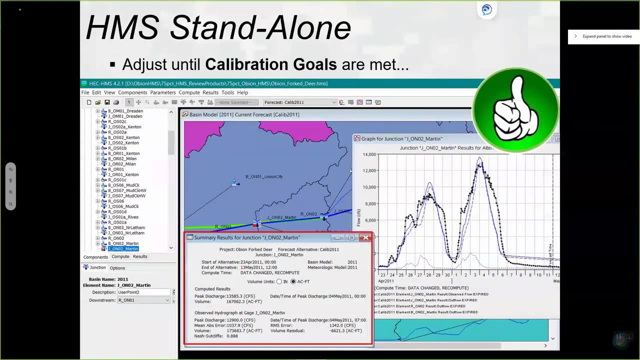 highlight the parameter column and then right click and select fill, and from here you can adjust by a number of factors to scale all the sub-basins at once. you can select the multiply by constant option and then okay, and then from here you can kind of just continue adjusting those parameters. 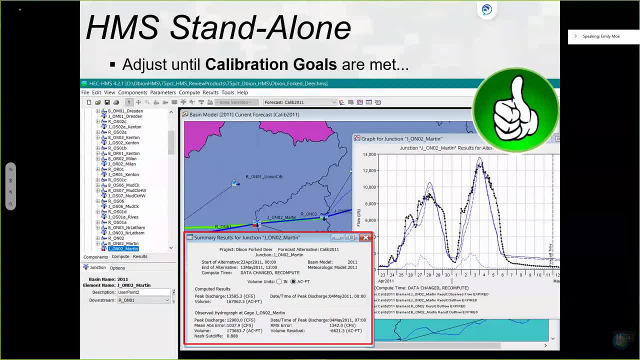 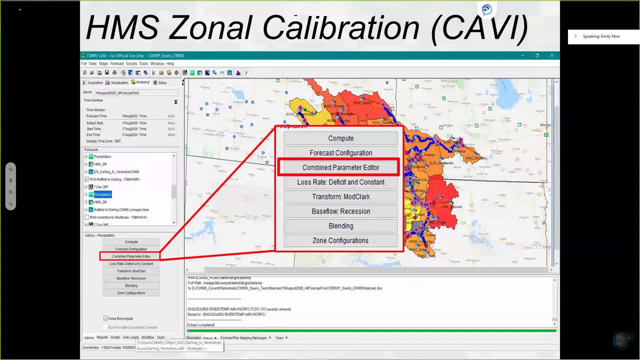 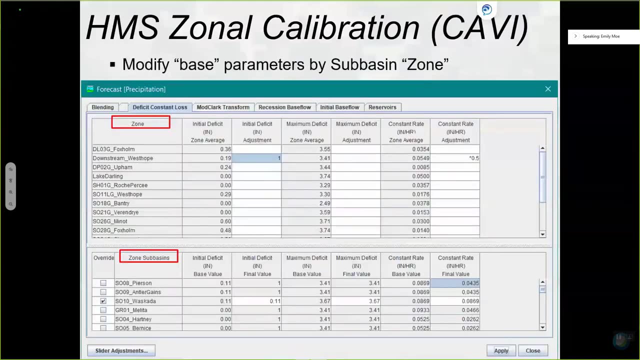 by computation point group until the calibration goals have been met. so another way to approach a calibration is to access the hms model from within the swim's cabi using the combined parameter editor. so this combined parameter editor, it provides a way for the modeler to adjust parameters. that 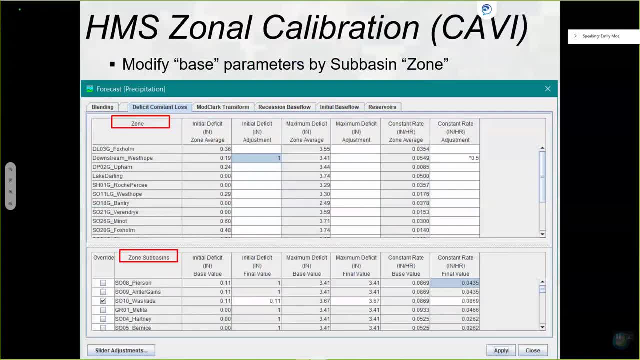 it provides a way for the modeler to adjust parameters. that also by groups of sub-basins, but in this instance those sub-basin groups are called zones. zones can be set up to include any group of sub-basins. ideally, each zone would be composed. 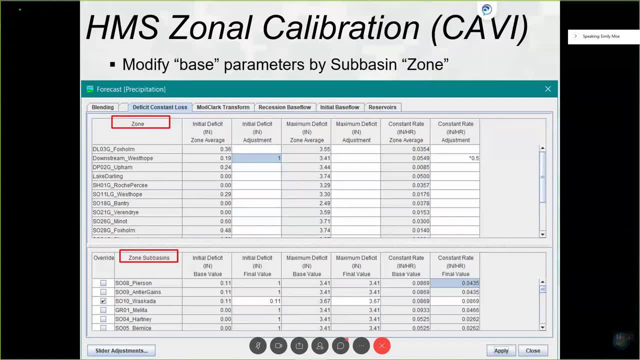 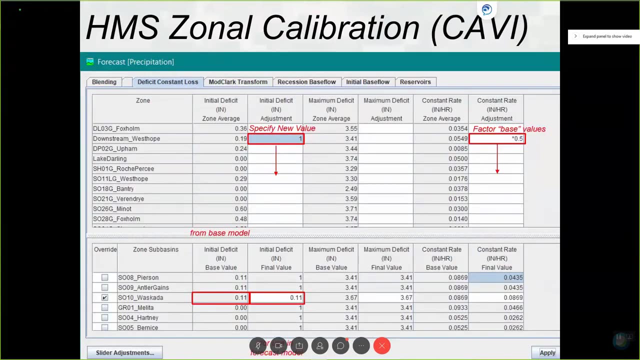 of sub-basins with similar characteristics and that behave similarly during rainfall events. one good way to approach setting up zones is by gauge, so similarly to how we selected the computation point grouping in the last example. so defining the groups of sub-basins within each zone allows the modeler to scale or modify the 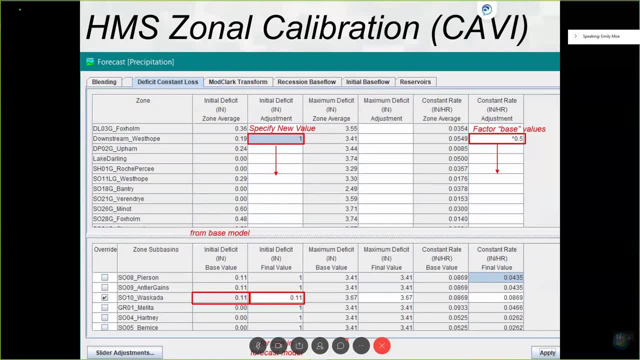 entire group of sub-basins in the same fashion all at once. so, for example, here in the top window we're working in the downstream west hope zone. since we have that row highlighted in the lower window, all of the sub-basins that are assigned to that zone are shown. 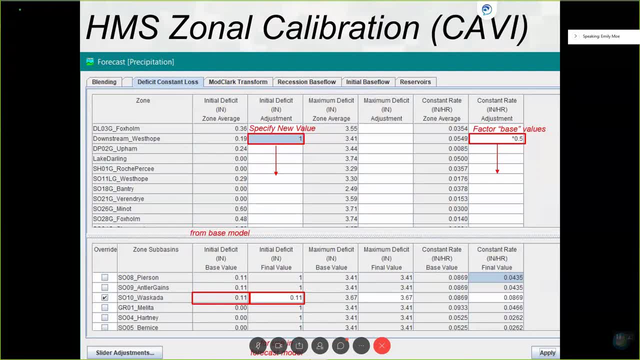 along with their base values of the loss parameters, and these base values within the cabi come from the original hms calibrated values. the combined parameter editor then allows the user to adjust these base values all at once within the entire zone, and this can be done by specifying a. 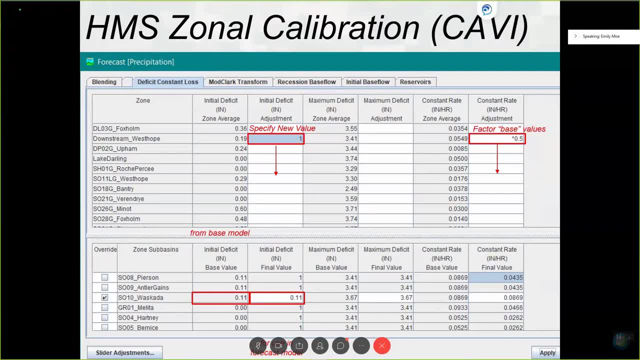 new value such as one inch on the upper example there for the initial deficit, or the user can factor those base values, for example, over on the right. we're factoring those constant loss values by 0.5, so we're cutting them in half and the adjustments that get made in the upper window are then reflected in the final value. 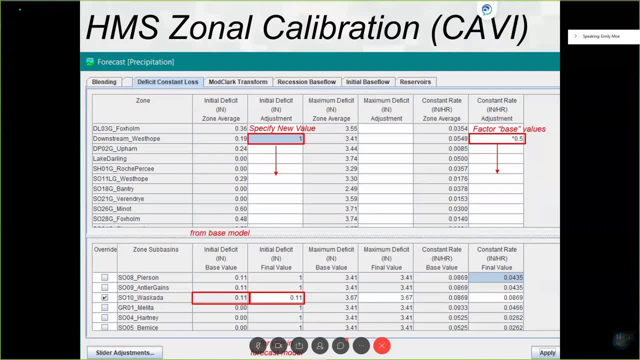 columns in the lower window, and these final values that are shown here are what will then be used to do the hms computations within the model when it runs next. the combined training editor also allows the override for a particular sub-basin, if you think that that particular 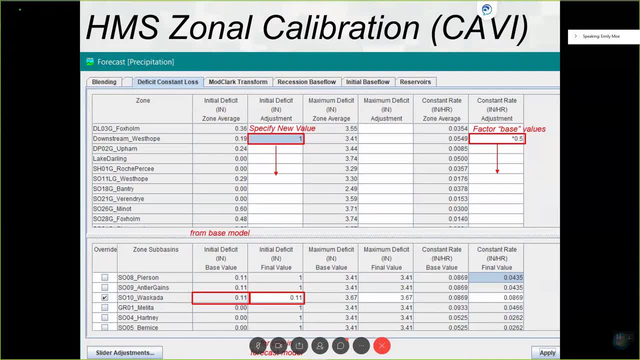 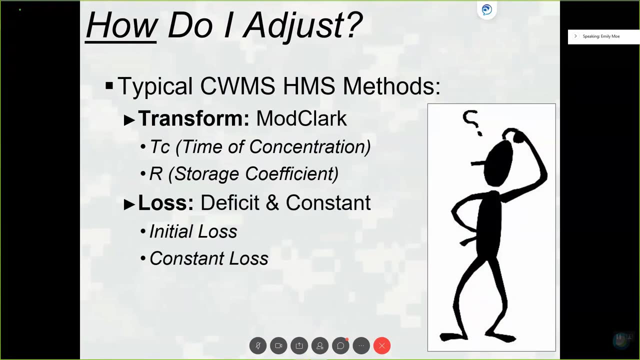 sub-basin may need additional individual adjustments, and this can be done by selecting the override box on the far left side of the lower window. so now we have calibration goals. we know where and how we might be calibrating the parameters, but how and which parameters do you? 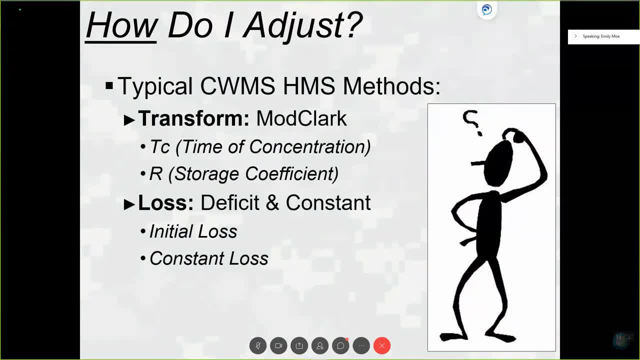 adjust during calibration. for this example, we'll look at some of the key calibration parameters from some of the most common hms methods that are used in swims models. this includes the mod clark transform method with tcnr and the deficit and constant loss method with the initial and 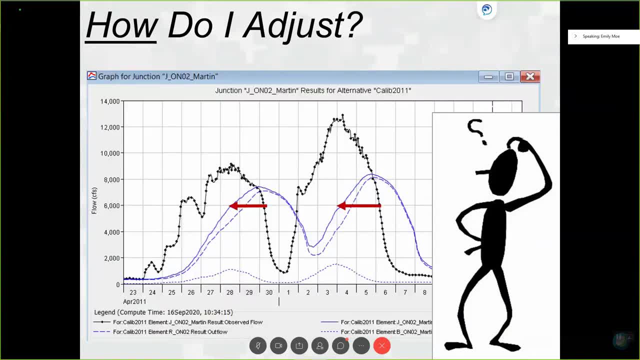 constant loss parameters. so when you're first learning how to calibrate in hms, modelers can often see the observed and modeled hydrographs and identify elements of the modeled hydrograph that you need to adjust and update to match- better match- the observed data. but it's hard to know which parameters that you might might start adjusting. 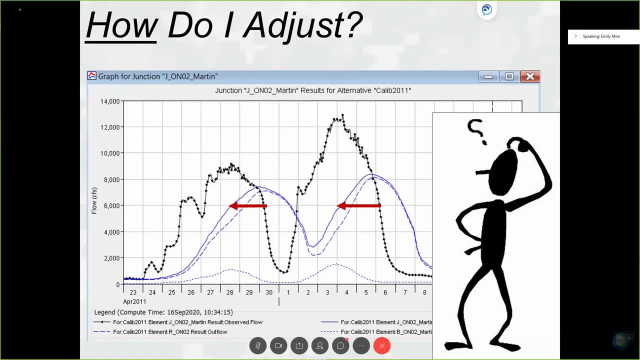 in order to to better match that observed data. so, for example, here we can see that the modeled results in blue are similar to the observed data. we've definitely got two peaks, just like the observed data in black shows, and we can see that the hydrograph needs to be shifted further to the 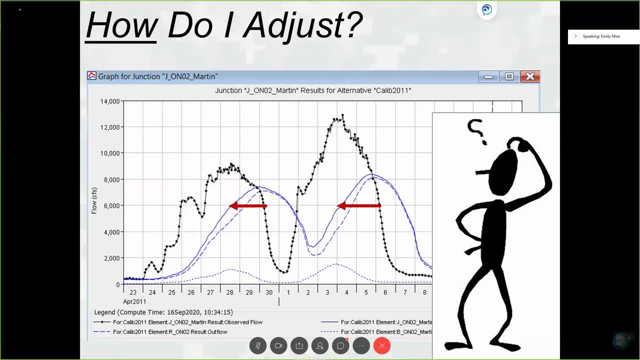 left. but when you're just getting started, how do you know which parameters to adjust to bump it further to the left and get the timing better? it took me quite a long time to really understand which parameters provide what responses and once i figured that out, i put: 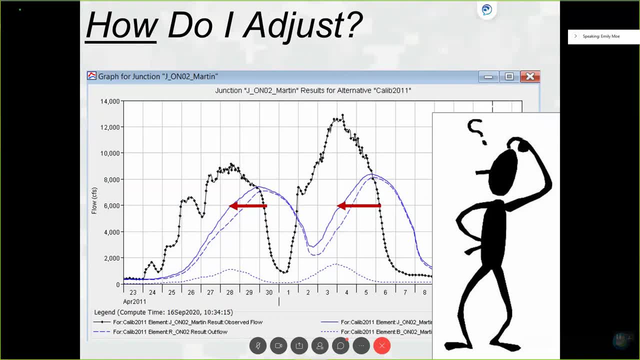 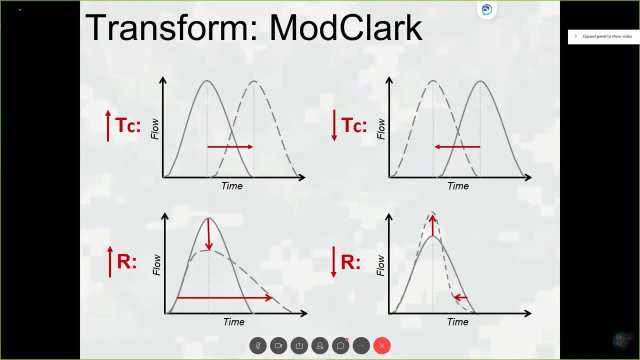 together kind of a cheat sheet that actually illustrates the responses of adjusting the different parameters. so the cheat sheet can be a really great reference to a new modeler to help them decide which parameters they might need to adjust and when. so for example, here we're looking at the mod clark transform parameters- we can see that increasing the tc values 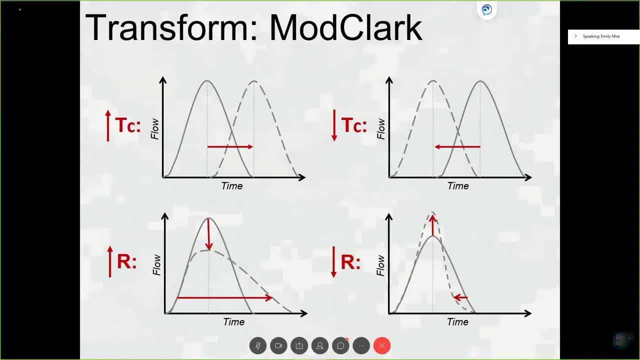 translates the hydrograph forward in time and decreasing the tc value translates it backwards. increasing the storage coefficient r increases the available storage within the subbasins, so it generally decreases the peak and attenuates the volume further out into the future. so essentially, if you it's the same volume throughout here, there's no losses you basically if you took a hand. 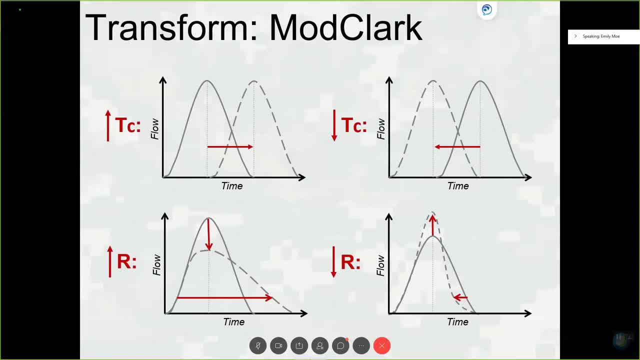 and just squished it down. that's kind of what increasing the storage value does to the hydrograph and in the opposite direction, if you lower that r value, it's kind of like pinching it. it reduces the amount of storage, so it drives up the peak and it brings the total event volume closer in. 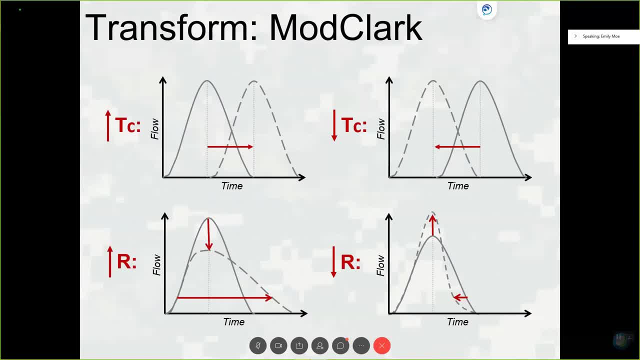 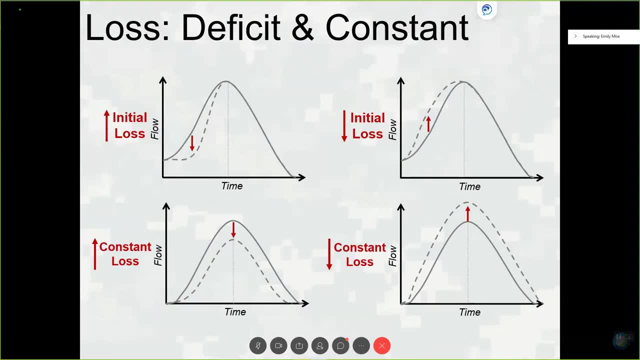 towards the and provides produces a senior or a pinched hydrograph like that. so for the deficit and constant loss parameter response examples, if we increase the initial loss, it indicates that the soil is dry and it has the capacity to take volume out of the system and that the volume loss is happening at the very 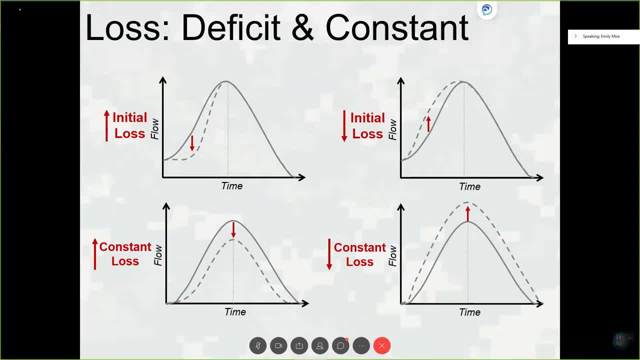 beginning of an event. so decreasing the initial loss indicates that there's less soil capacity, perhaps it's already totally saturated and therefore more volume goes into the initial part of the hydrograph. the constant loss rates affects the magnitude of the entire hydrograph throughout the whole event, so increasing that constant loss pulls more volume out of the. 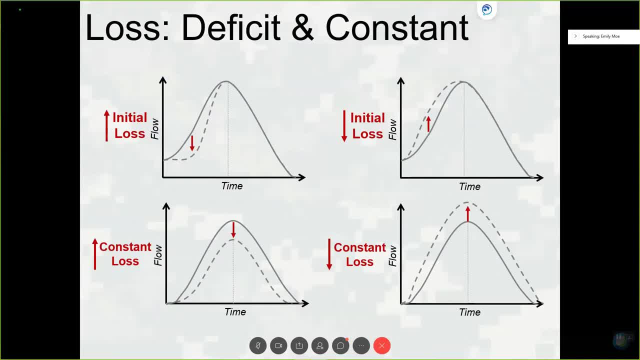 hydrographs, which reduces the overall peaks and decreasing the constant for relying on our water. normal microplastics will only reduce certain volumes longer and make right the whole event. the being in the system thus rates has the opposite effect and increases volume and peak magnitude. so the the cheat sheet parameter response diagrams kind of provide a good idea of which parameters. 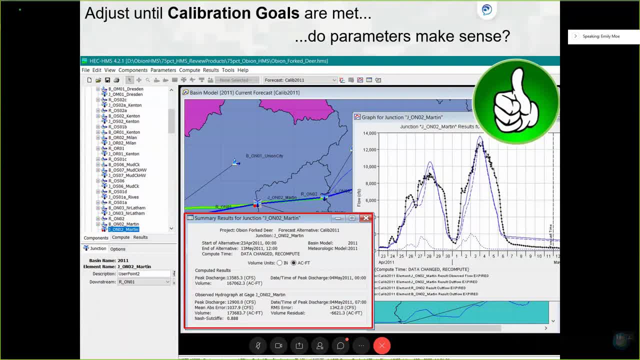 might require adjusting throughout calibration. the goal is to kind of just continue those adjustments, one at a time, until the calibration goals have been met, and don't forget to stay within realistic ranges of each parameter. certainly make sure to revisit the final calibrated parameters and ask yourself: do these make physical sense for the basin? if not, is there a reason? why is it like a? 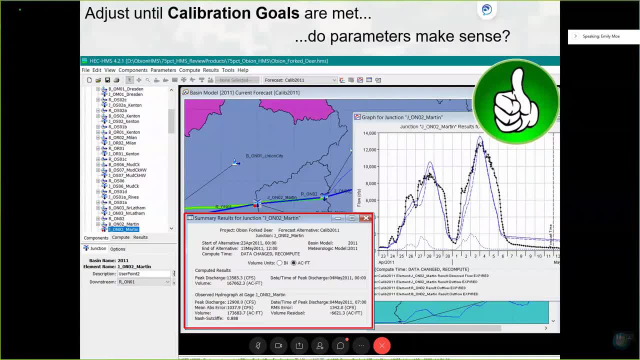 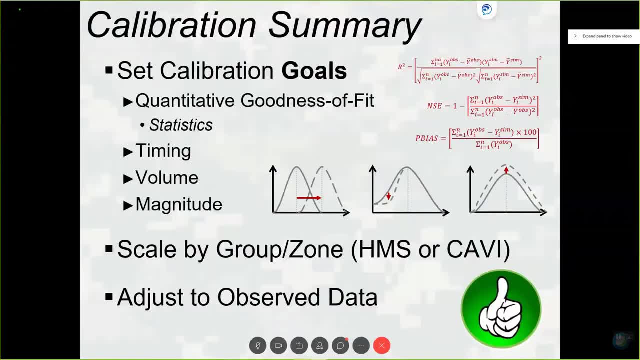 highly urbanized area, or is there an extreme soil condition or something that would explain that? so, in summary, it really helps to set calibration goals that are reflective of the scope of your project. scaling the group by group or zone is a handy way to calibrate several sub basins at once. 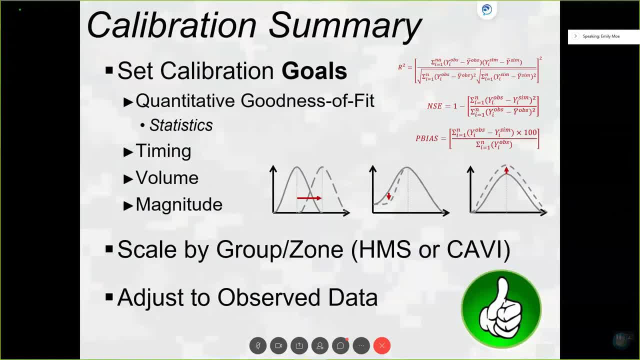 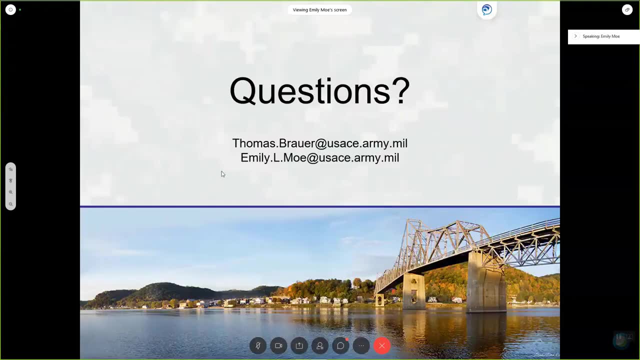 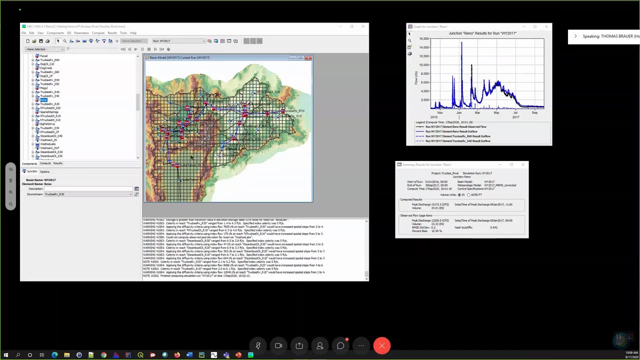 and still maintain stability, and you can also use the tool that is available in the tool box to determine which parameters might require adjustment during calibration and consulting your parameter response cheat sheets can be helpful to new modelers to determine which parameters might require adjustment during calibration. and that that is really um. those are really all the tips that i had, so, yeah, let's just. 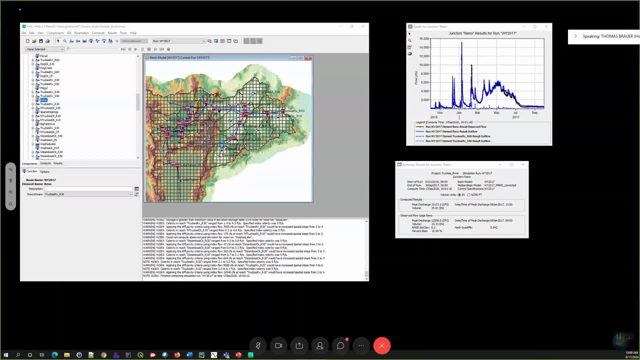 talk a few special cases and tools coming. i'm coming from the development perspective and um, but we'll just show you some of the things we have now. so, uh, the the graphs and the summary tables that we show and we have in hms. they're great. one of the limitations is they're for a single point. 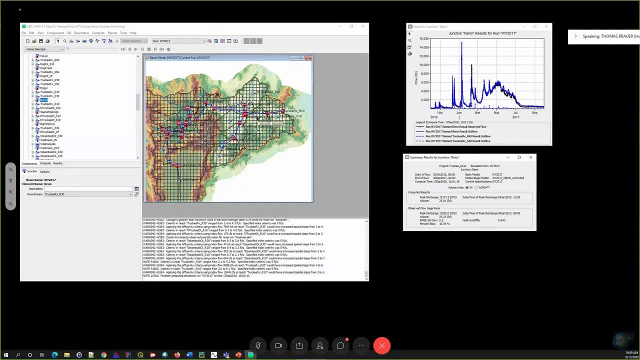 only so i've pulled up. this is my marbles truckee river project and i pulled up some results for reno. so a common thing that we get asked is how to do these things for the entire modeling domain, and one of the things we took a step to do. 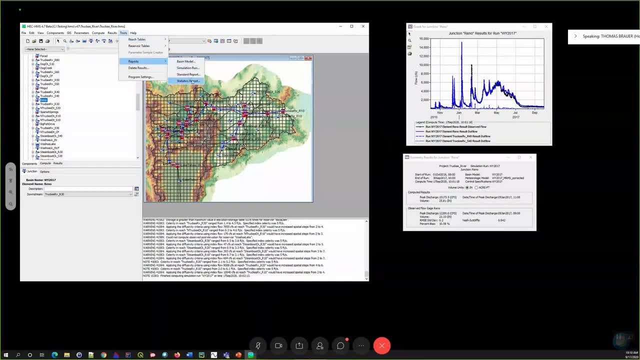 is add this statistics report, and so it's in is introduced in 4.6. so report statistic reports. i have my runs selected: uh, water year 2017.. so, see, i'm just gonna save this out. all right, let me generate it. and so what this is going to do, is it? it's going to loop over all of my calibration locations. that. 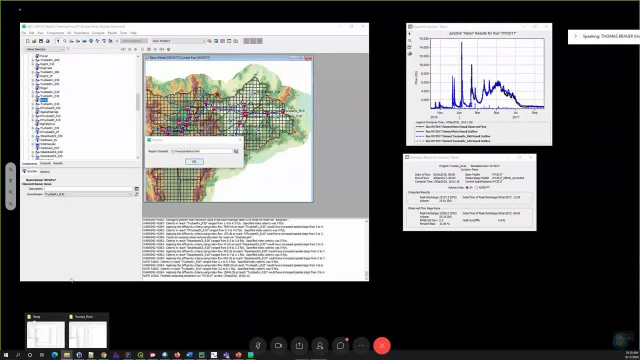 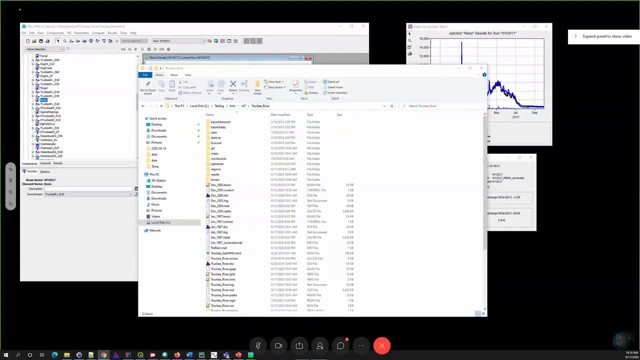 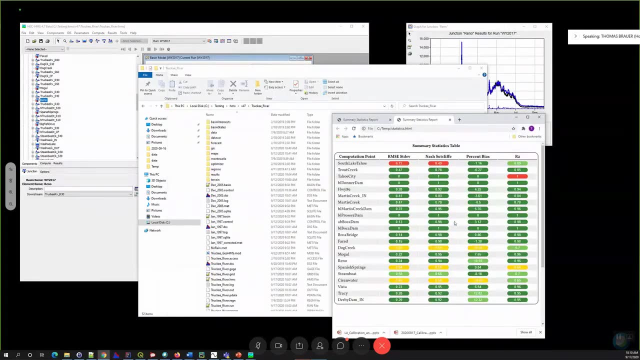 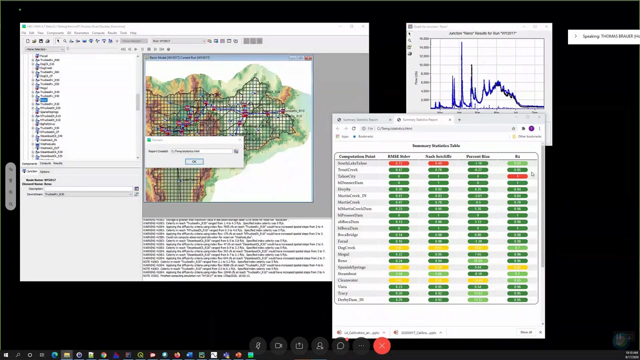 flow and it's going to run statistics on all of them. So what I should get is a nice report that looks like this: So for each calibration location, you can see I have the computation point and then I have my statistics- all the ones that we went over. So that's nice. It's something we often do as part of. 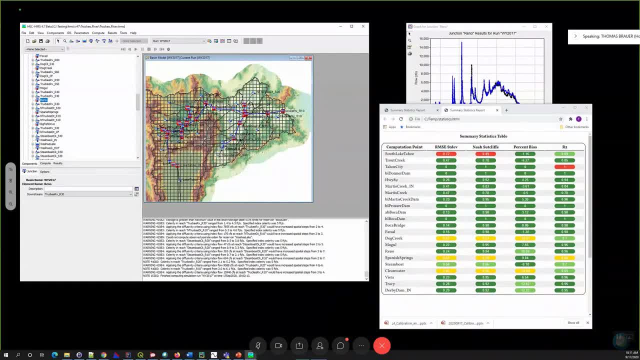 the reporting process, so this just streamlines that. I know for ongoing model calibration. you're doing calibration runs and you want to see statistics a little. it's a little cumbersome right now. One of the things that I'd like to see in the future is for this to become a table much like 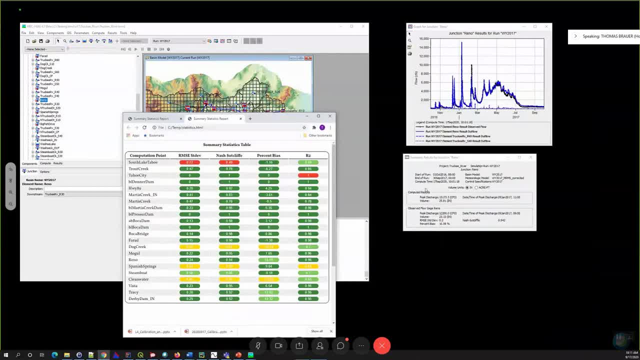 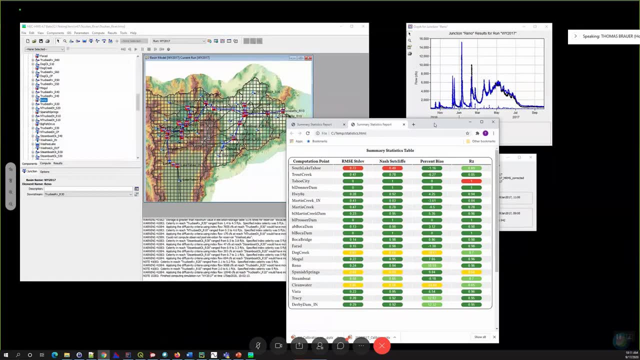 this right here, and so with every run, simulation run, you do it automatically updates. So I guess we always have at AGC we frequently do our sales pitches. so that's one if you think that would be cool or you're interested in something like that. 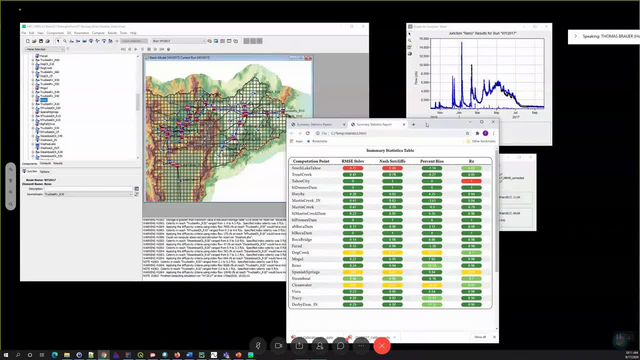 You can work with WMIST or somebody to find a way to fund it. Another thing that we talked about is maybe color coding some of these locations in the model themselves, based on how the calibrations come out. So this gives a spatial notion. There's all these different spatial points, the spatial 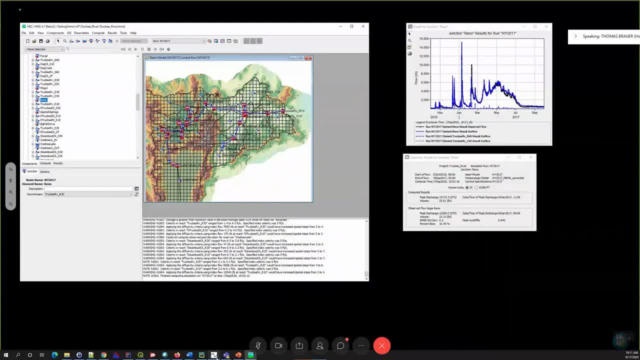 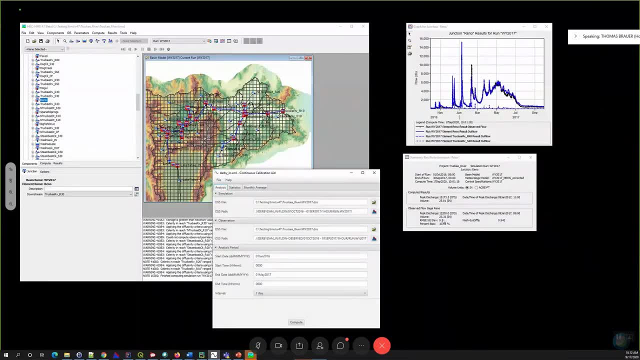 notion of how the model is calibrating. Another kind of special use case is that the reality is is that these statistics that are calculated in HMS are for the entire duration of the simulation period and they're calculated at the simulation time interval. So often people 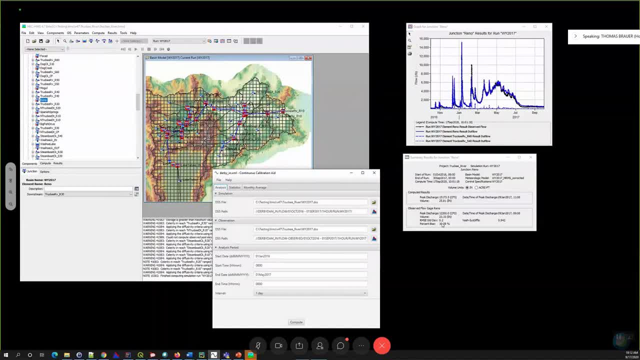 want to adjust the computation interval for the statistics, but something different than the simulation time interval. What we did, a kind of like a annual volume type study in the Northwest, and so we we had, I think we had like hourly flow data, but we've only had daily precip data, and so we kind of 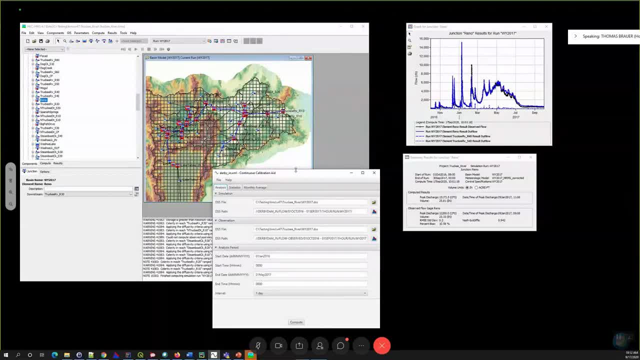 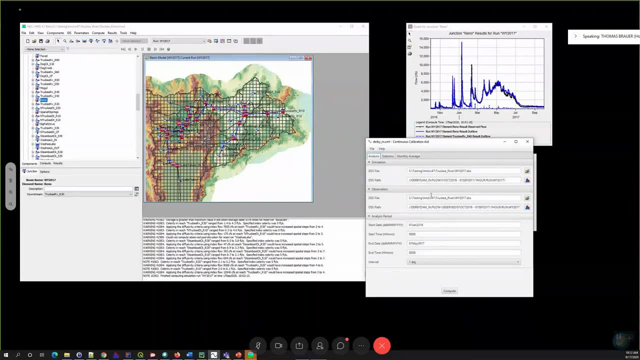 wanted to normalize the statistics to the day, And so what we developed for that case is this calibration aid. you might have seen it's kind of gone around as well, and so what this allows you to do is compute those statistics that whatever interesting Sort of an unit of noってる, no dues, and we had a delicious 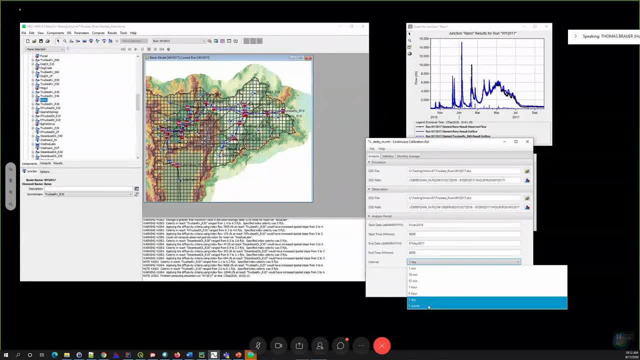 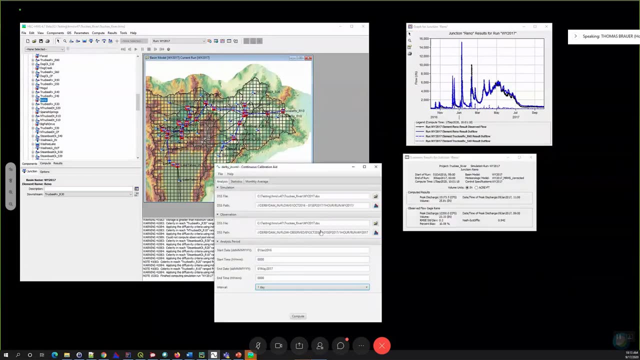 so you can't even run an HMS model two months a time. stop. but if you wanted to compute, say you know reservoir impuled volumes to the month or how the statistics compare, and you have that option here and then the other thing that you can't really do with HMS but you can push you to do, this tool is just: 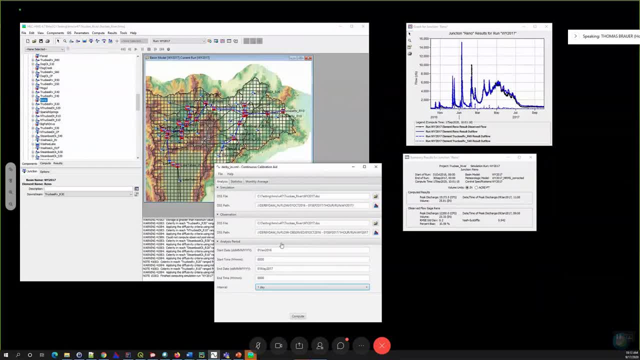 adjusts the of the statistics calculation. so often for, like a snowmelt water year, we're running from October all the way to September, but the real focus of the calibration is between January and May, June, July, and so I can do things like cut the time window down here, so I just focused the statistics on to the period. 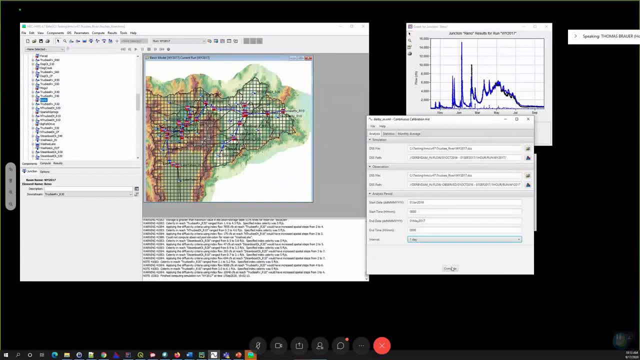 that we're interested in, which I did here in January and May, so I can compute those statistics here, the statistics table. once again, this is just a point location- you can open up a bunch of them, but just a single point- and the tool and then I can view these monthly average, how the volumes compare. so those are. 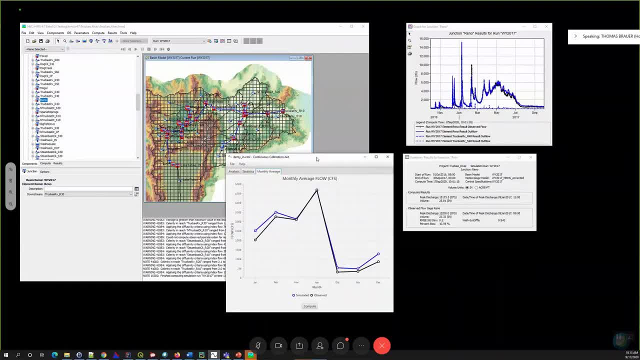 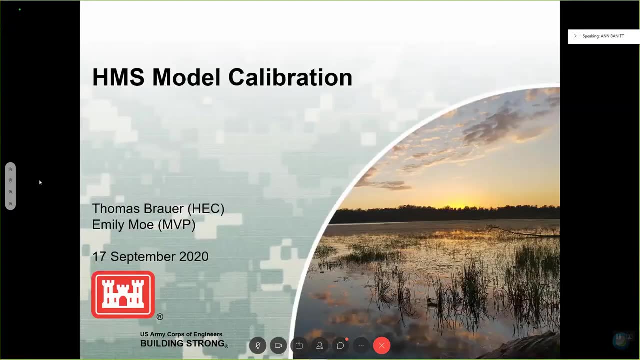 just a few extra little tools you might be interested in if you situation. you did all right. so with that I think we can go to questions. I'm gonna ask you a couple questions that have popped up on my screen. I think some of them are interesting to everyone, but some of them aren't. so one of the questions is, I think, Tommy. 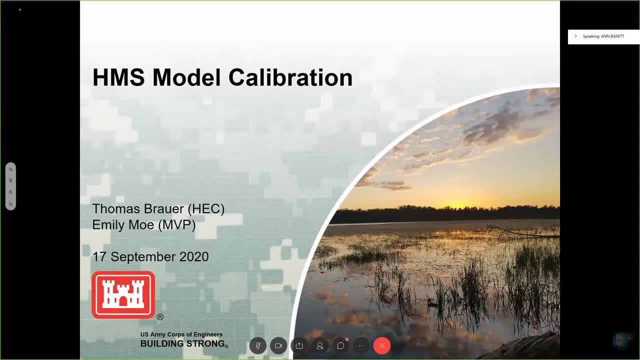 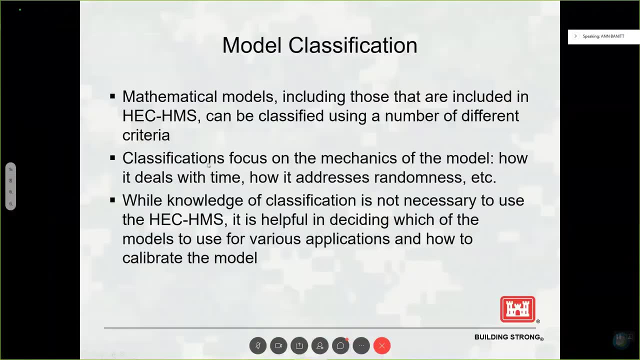 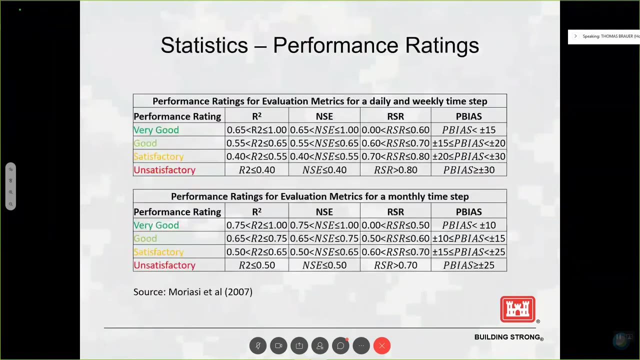 might be answering this one. do the summary statistics have published standards for time steps smaller than a day, or is it acceptable to use the one values for smaller time steps? yeah, let's take a look at that. so here's the table right. so the published. you see there it says daily or weekly time step. now one. 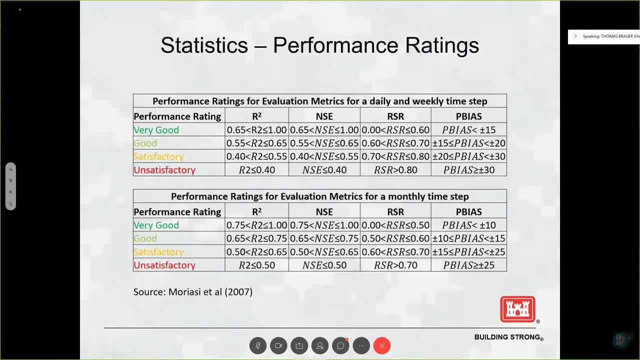 thing that you'll notice is, as the time step decreases, these ranges only get more relaxed. so we just went from you know, doing monthly time step, good, it's 0.75. you're doing daily, good is 0.65. so what I usually tell people there: there is not published ranges for that, although there has. 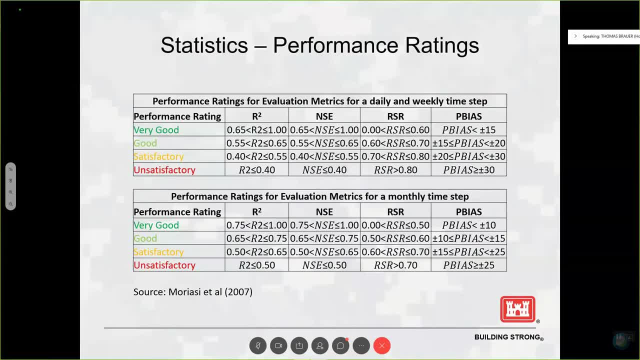 Moriarty in our group have put out another paper to, so it's worth consulting there. but I think the last time I looked it wasn't. they didn't try to publish anything for less sub daily. so what I usually tell people is: if you can meet this criteria, you're good, because these things are going to be so good. 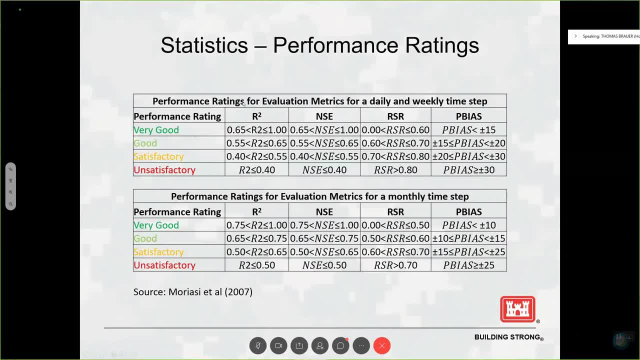 only getting more relaxed if you went down to a day, you know it might be something like 0.55 or something if you extrapolated this. so I always tell people: just shoot, shoot for the daily criteria and if you're doing, you know if you're running your statistics at the hourly level you'll be good if you're. 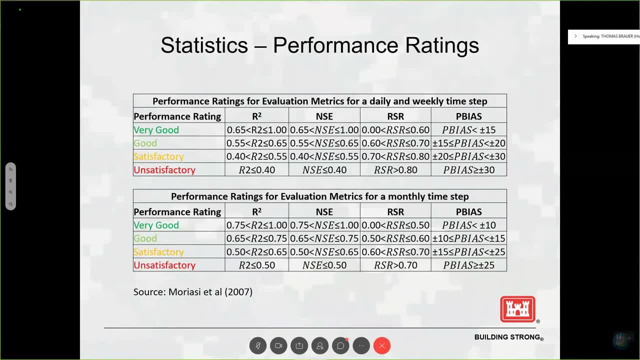 not good. you're gonna have to do some justifying. so if you're at you know, point point six, zero here for your hourly, then I think in your report you'd have to say just some reasons why you know. but if you hit this, no one can ask. 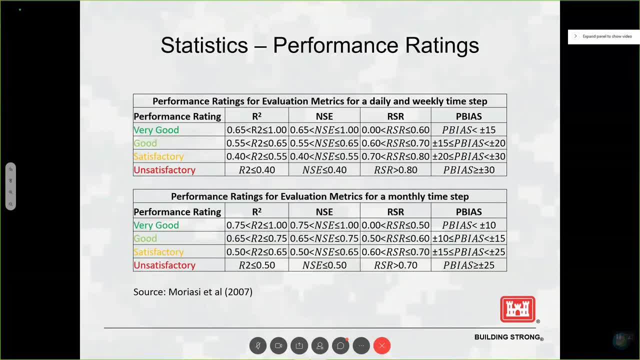 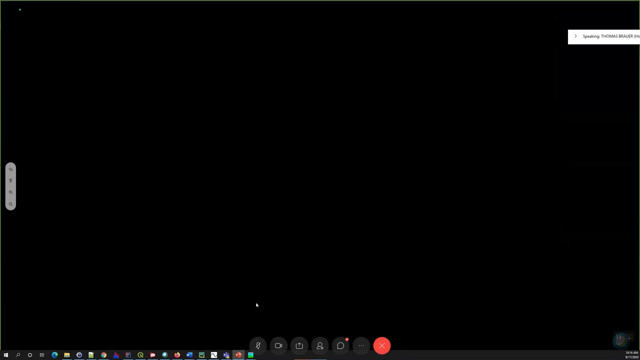 questions then time. are there ways to like cut and paste- calibration incorporates setting calibration goals within HMS- to avoid having to manually type them into a spreadsheet? or you talked about having your report, but can you copy and paste values from some sort of file? I mean, yeah, if you're using a spreadsheet, you're kind of acknowledge. 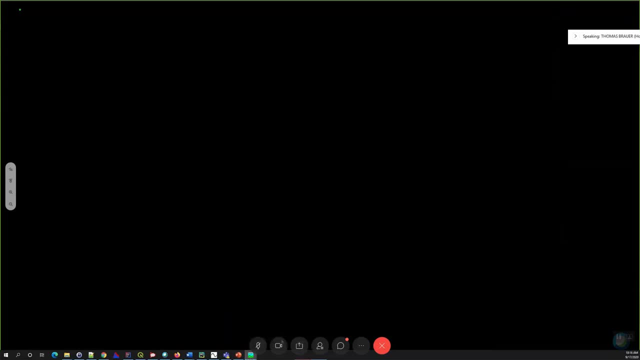 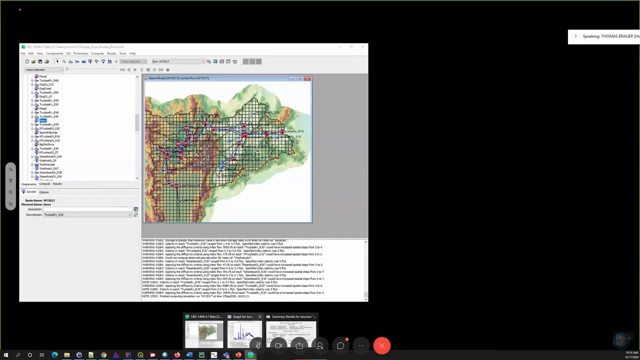 it's going to be a bit of a manual process trying to open HMS. you get this guy back over, pulled it all the way. I don't know how well these table copy and paste, but yeah, there's not. I'm not able to like grab that, so it looks like you'd. 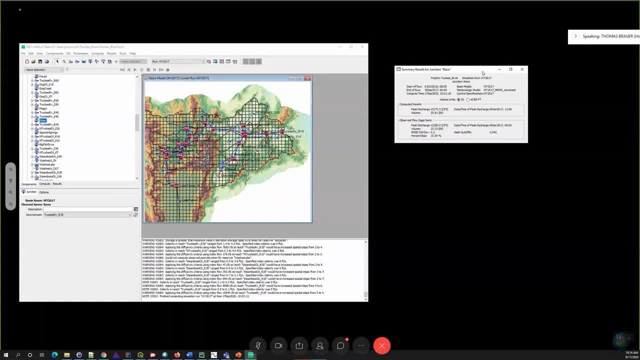 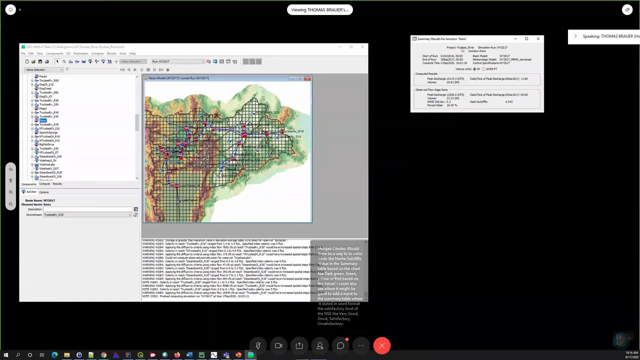 have to type that in. yeah, these are all things that could get better. and development I think we should work on as a community. you know, modeling community and future is creating some sort of table and adding like a clipboard option where we could grab everything on the table. okay, super, um, we have a question here. when you're 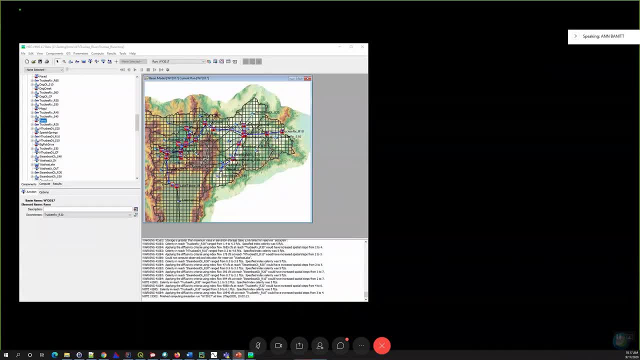 using Clark's method. often the ratio of R over P C plus R is regional constant. are there any plans to have HMS compute that ratio instead of computing it yourself outside of HMS? yeah, that's, that's a. that's a good one, and that is true often as our GCR what's our relationships? it's not. I don't know that. 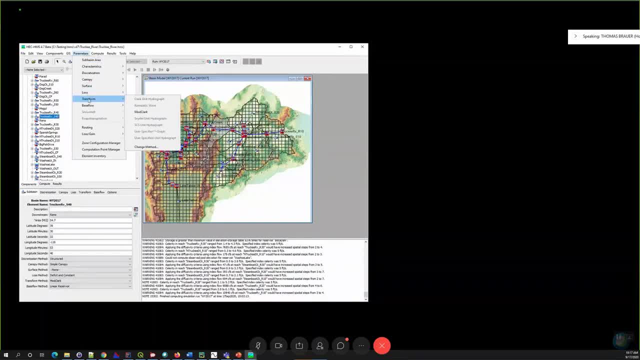 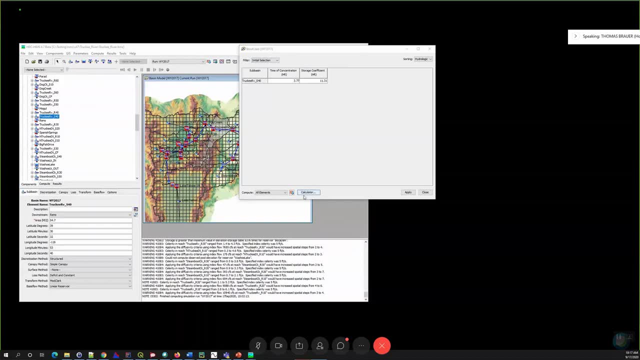 we can do that exactly. right now there's something in development. let's see if this version of HMS- I have a development version pulled out there, so this is a new version of HMS. so this is trying to work around Webex. let me grab the window. so this is the new expression calculator. so you can see I have a global editor. 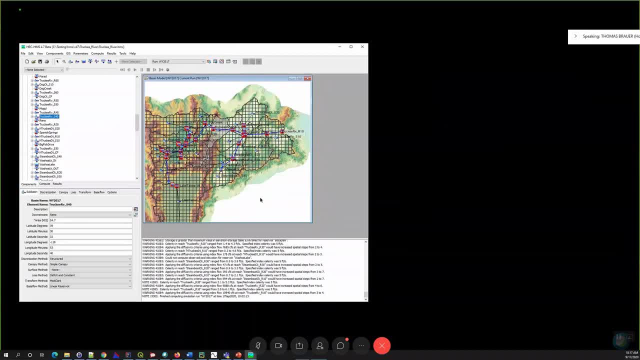 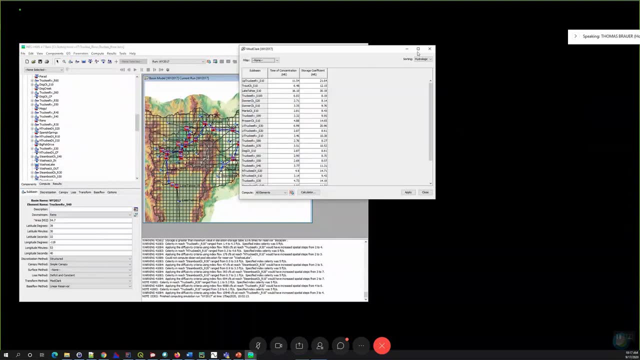 where I can. well, I have a single selection. let me close this, not select a sub-basin. so I just have a sub-basin selected, only these: transform mod Clark. so now I should see all of my TC and ours for all my sub basins, and then I 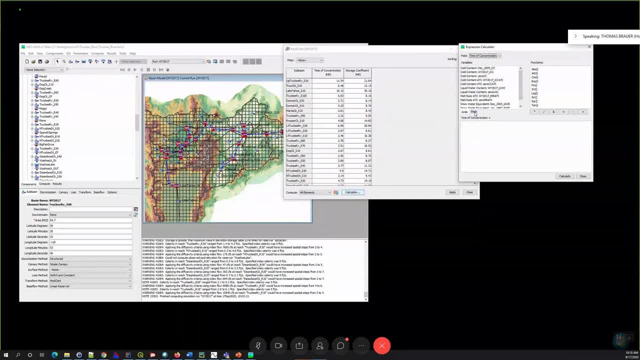 have this calculator and what I can do is I can calculate a time of concentration for all sub basins. now there's the one thing that's not in this version. that will be soon, and I can. I can do calculations based on grid better in my model, so I can sample those grids. 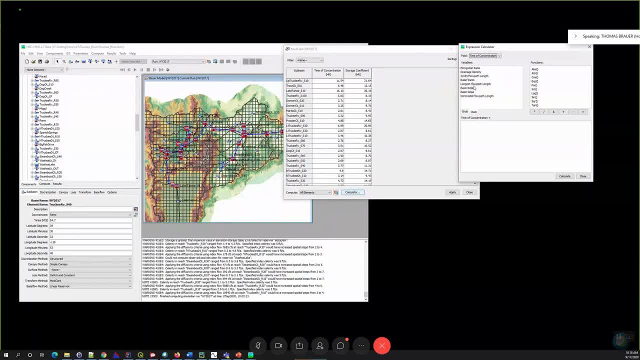 I can do calculations based on statistics. so things like long a slow path of my time of constant, let's just try it. real quick time of concentrate, or long a slow path, that's a good one. this is a dev version, so hope it works actually. no, I know, I haven't. well, that. 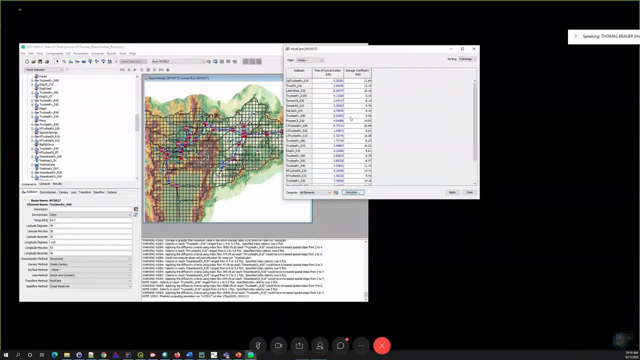 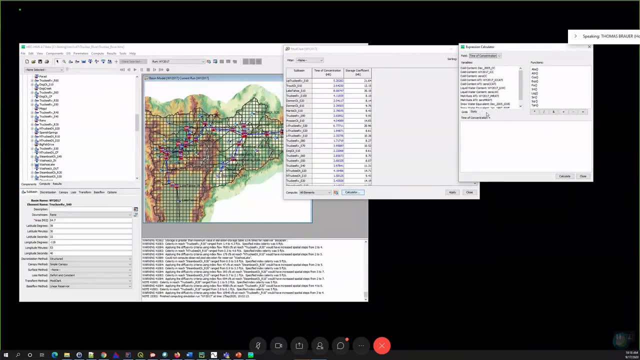 was actually pretty fast. so there you can see I've calculated my TC. the next piece that we're going to add is a tab called field, and what field allows you to do is look at field better to the left and right of the column you're trying to. 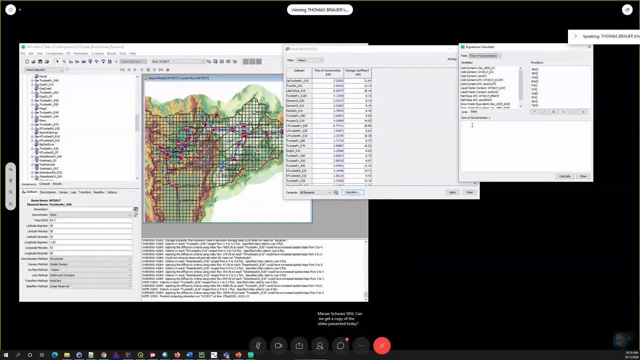 calculate, and so I could potentially put in this box down here the any format I want for calculating a particular field. and so then the next question that people ask it's like: are you going to have standard equations built into this calculator? I think that's a great idea. so R over T, C plus R is something that 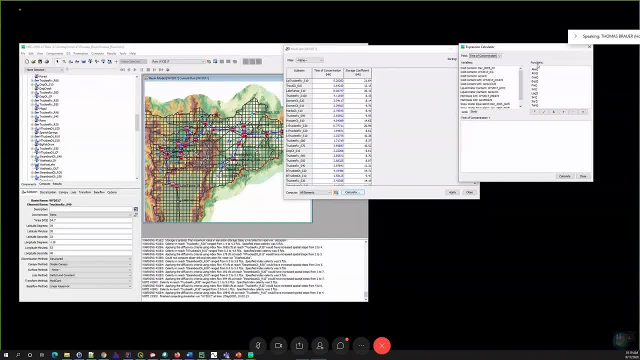 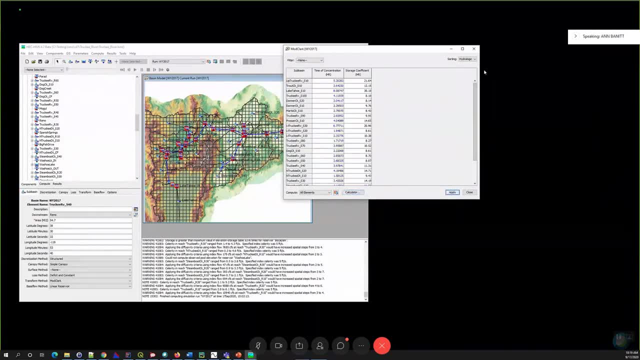 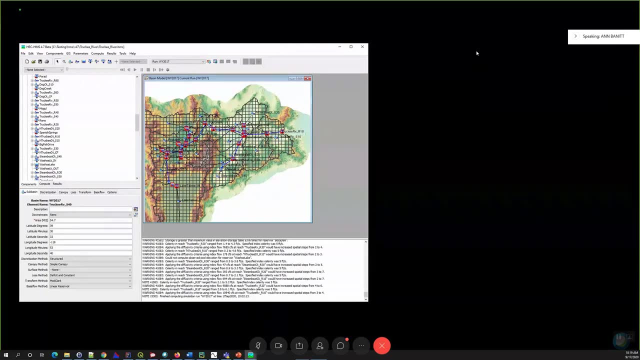 we could enforce and the expression calculator. all right, but the at times when you review models, it's nice to have some of the physical parameters that were used in developing the original model. for example, knowing the length and slope of the routing reach can help make a determination. if the routing parameters were reasonable, are they computed as? 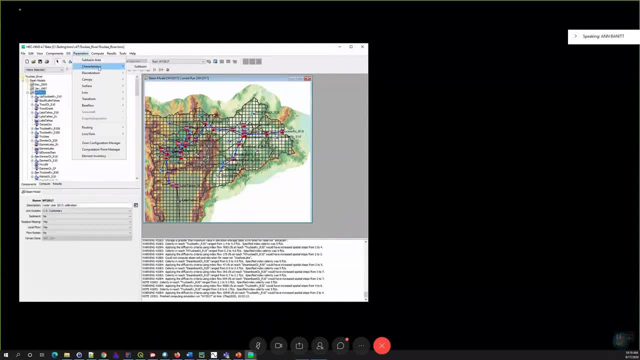 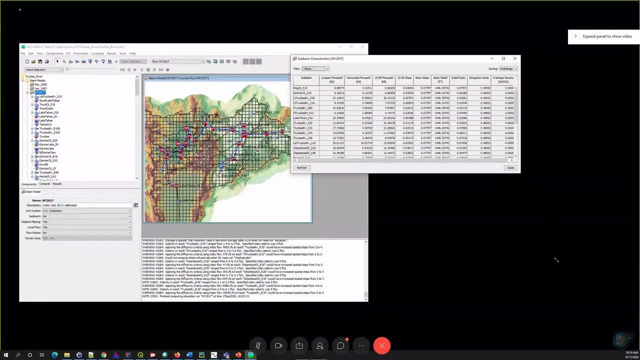 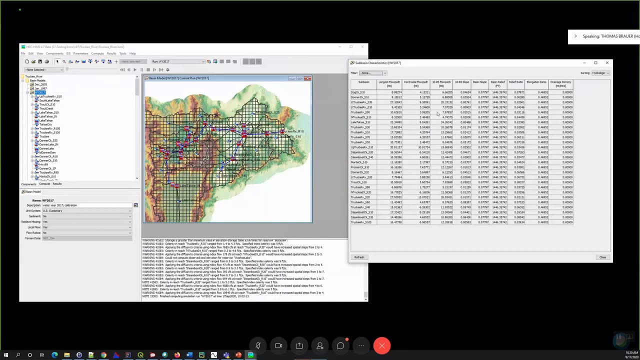 part of the DOHMS process, and can they be stored as metadata somehow tied to elements in the model? okay, so I think you're asking something similar to what we've recently added as well. we have sub-basin characteristics, and so you're asking something similar to what we've recently added as well. we have sub-basin characteristics, and so 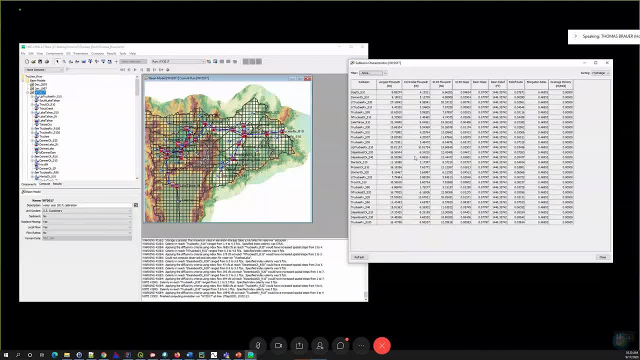 you're asking something similar to what we've recently added as well. we have sub-basin characteristics and so I just showed the expression calculator which I just showed, the expression calculator which references these characters. this is all. I just showed the expression calculator which references these characters. this is all devs to well, it'll be in the 4.7 beta release. it's. 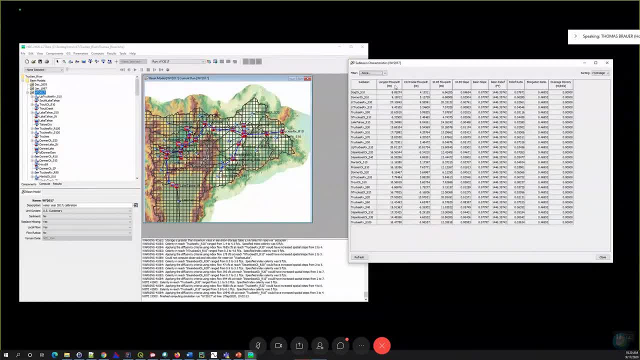 references these characters. this is all devs to well. it'll be in the 4.7 beta release. it's soon to hit the streets, but we've soon to hit the streets, but we've implemented statistics or characteristics, implemented statistics or characteristics for the sub-basin. everything you see here. 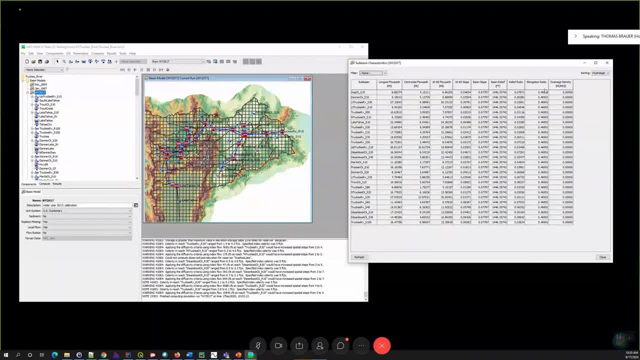 for the sub-basin, everything you see here: longest flow path, some slopes release longest flow path, some slopes release things like that. and we actually have things like that and we actually have implemented in the code some reach implemented in the code, some reach characteristics. so things like length, slope. 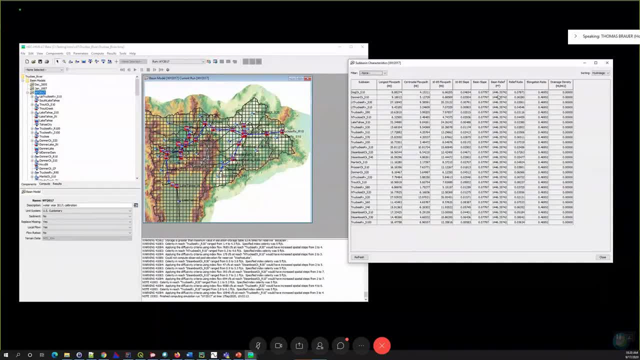 characteristics, so things like length slope release characteristics, so things like length slope, release of a routing reach I need. I release of a routing reach I need. I release of a routing reach I need. I still need to hook that up in the. still need to hook that up in the. 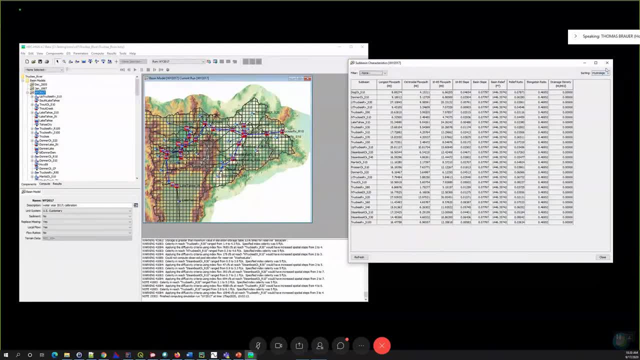 still need to hook that up in the interface. it'll look very similar to this interface. it'll look very similar to this interface. it'll look very similar to this, and once we have these statistics, then and once we have these statistics, then and once we have these statistics, then they're accessible through that. 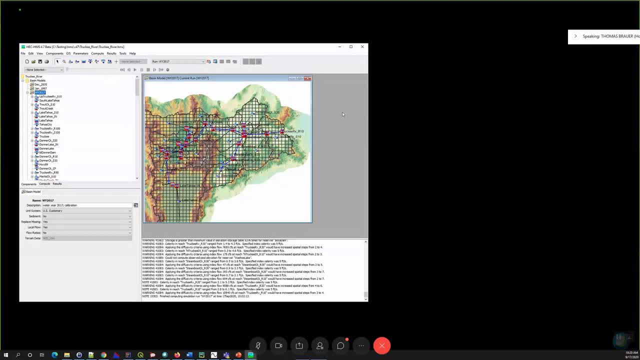 they're accessible through that. they're accessible through that expression calculator that I just showed. expression calculator that I just showed. expression calculator that I just showed that can be used in the global editors. that can be used in the global editors. that can be used in the global editors to help parameterize the model. pretty, 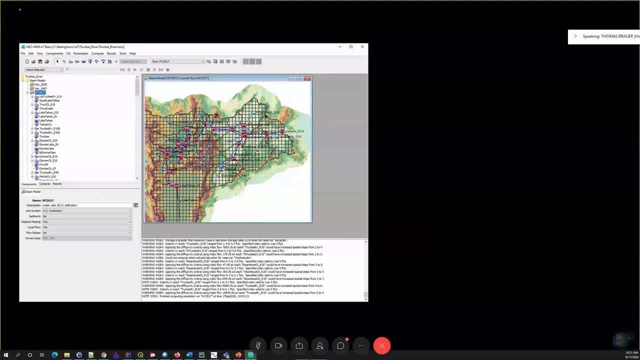 to help parameterize the model, pretty. to help parameterize the model pretty. exciting time. yeah, I'm excited about it. exciting time, yeah, I'm excited about it. exciting time, yeah, I'm excited about it. these are good questions because this, these are good questions. because this, these are good questions because this has been my life for, like the past three. 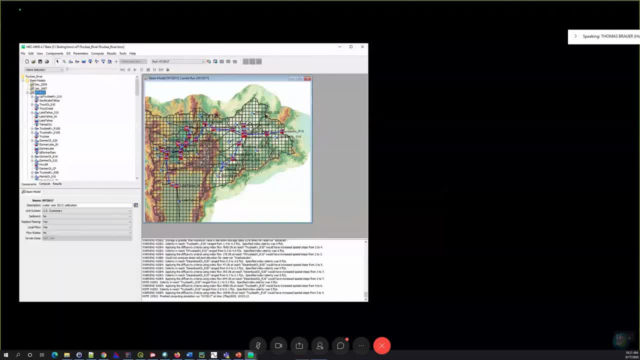 has been my life for, like the past three has been my life for like the past three months at least awesome. okay, here's months at least awesome. okay, here's months at least awesome. okay, here's another. I guess you have just a few more. another, I guess you have just a few more. 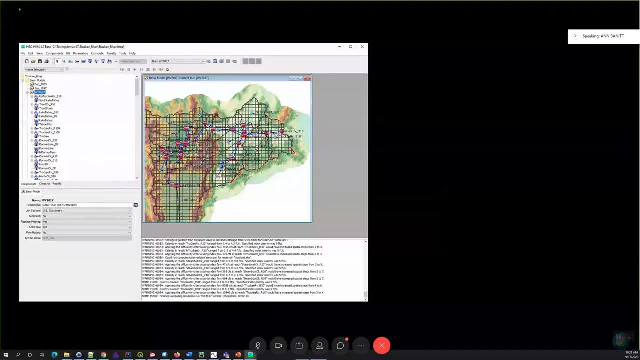 another. I guess you have just a few more minutes. heroes, he's wheeling through minutes. heroes, he's wheeling through minutes. heroes, he's wheeling through them until we get the buzzer. but um is them until we get the buzzer. but um is them until we get the buzzer. but um, is there a way to color code the Nash set? 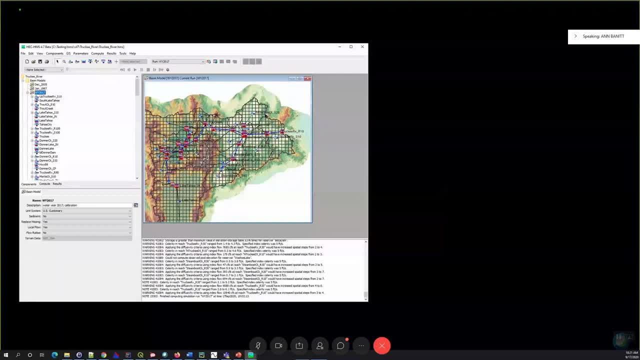 there a way to color code the Nash set. there a way to color code the Nash set clip value in the summary table based on clip value in the summary table. based on clip value in the summary table based on the chart like dark green, green yellow. the chart like dark green, green, yellow. 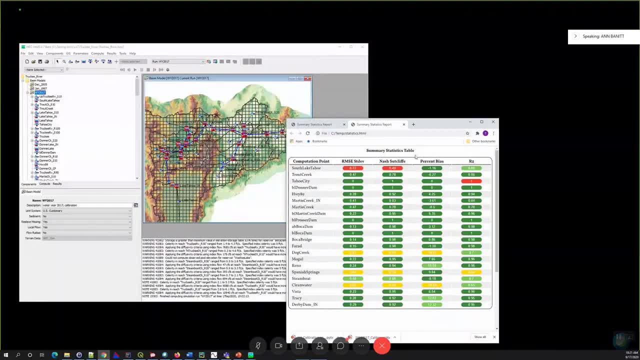 the chart, like dark, green, green, yellow, red based on the value. can also see red based on the value. can also see red based on the value. can also see where it'd be good to input to the, where it'd be good to input to the, where it'd be good to input to the summary table, where it's stated in word. 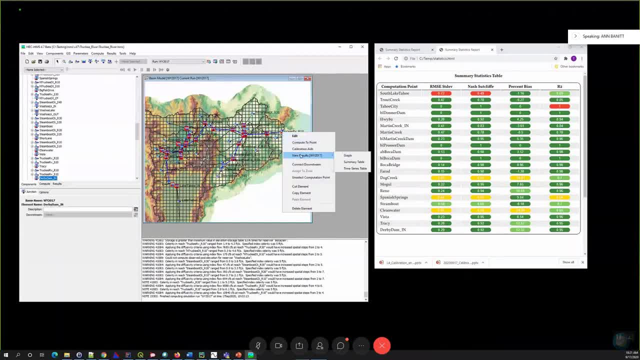 summary table where it's stated in word. summary table where it's stated in word format: the satisfactor level: like Nash format. the satisfactor level: like Nash format. the satisfactor level like Nash set clips: very good. good, satisfactory set clips very good. good satisfactory set clips very good. good, satisfactory factory on satisfactory. okay, yeah, yeah. 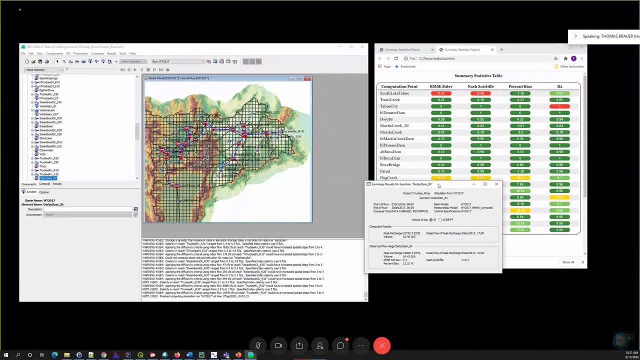 factory on satisfactory. okay, yeah, yeah, factory on satisfactory, okay, yeah, yeah. so a qualification of the table- good, so a qualification of the table good, so a qualification of the table good. questions we've considered doing that and questions we've considered doing that and questions we've considered doing that. and one of the things that always comes up: 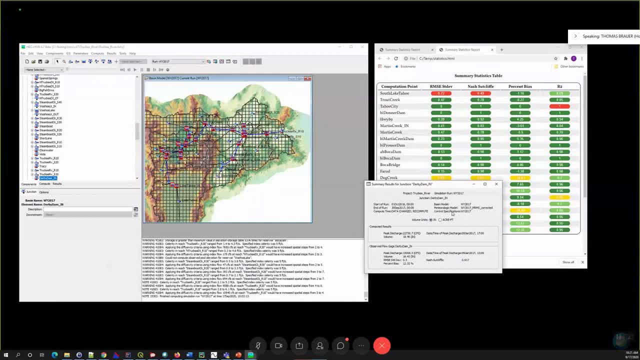 one of the things that always comes up. one of the things that always comes up because it can be done and should be done, because it can be done and should be done, because it can be done and should be done. at some point the consideration, though, at some point the consideration though. 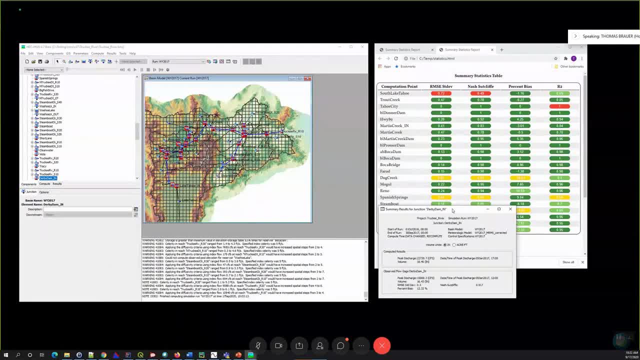 at some point. the consideration, though, is that we need to give the we want to, is that we need to give the we want to, is that we need to give the. we want to give the user some control over those, give the user some control over those, give the user some control over those ranges and color codes, and things like. 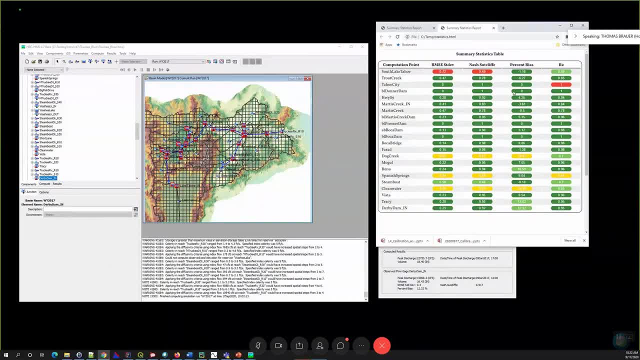 ranges and color codes and things like ranges and color codes and things like that. so with this statistical report, i that. so with this statistical report, i that. so with this statistical report, i did just use the moriarty values and did just use the moriarty values and 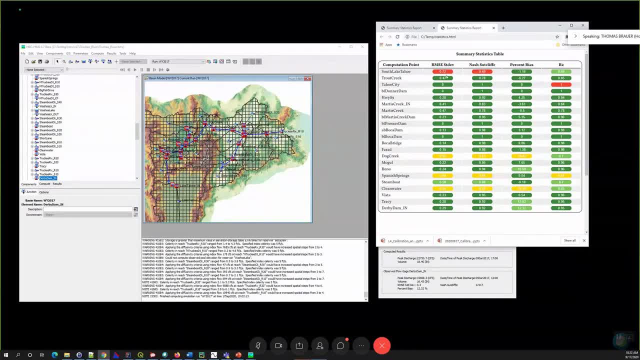 did just use the moriarty values and ranges and colors, ranges and colors, ranges and colors, and, and and documented it. so i said: when you run, documented it. so i said: when you run, documented it. so i said: when you run this report, this is how it's going to. 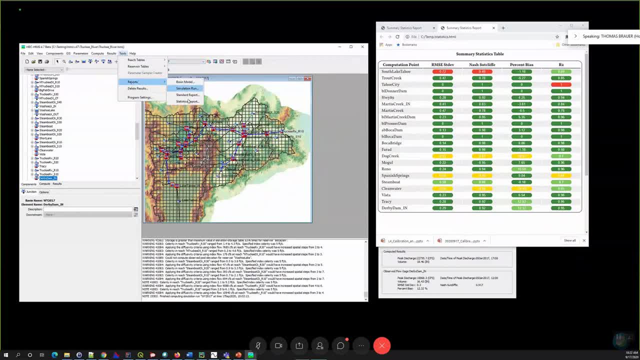 this report. this is how it's going to this report. this is how it's going to look, look, look, now in the future. i would love for this now in the future. i would love for this now in the future. i would love for this editor, editor, editor- to give the user some control. so what? 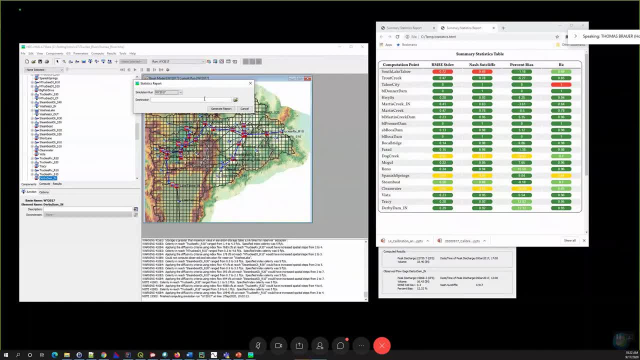 to give the user some control. so what? how do you want to then? and certainly one of the default options could be the moriarty ranges. but i think we need to give the user some control, because different circumstances dictate, you know, different needs, and so for the user, you say, hey, these are the bends. i want to put my statistics. 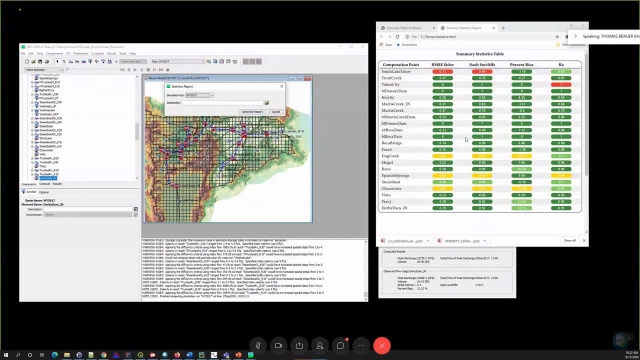 in and these are the color codes that i want to use. i think somebody already said i'm colorblind and this table's hard for me, you know. so things like that, um, give the user some control over that um, and i definitely, like i said i i would love to see this. this is just html table that we're. 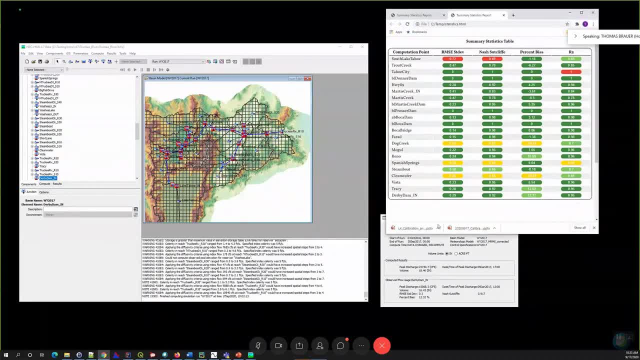 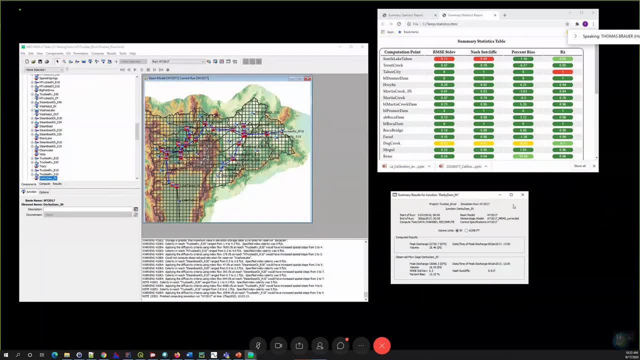 writing out at output. but i would love to see it as a java table similar to what we see here, that live updates, and maybe there's some user options or buttons up here where they can start to color code different pieces of it. all right, awesome. another question says one of the early slides indicated bad. 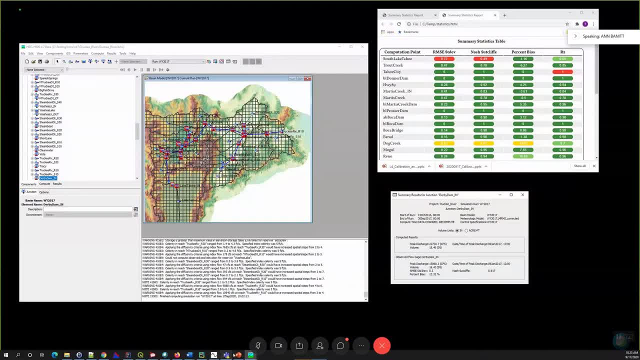 rainfall is being one of the biggest reasons for calibration difficulties. if you have several storms but the rainfall is questionable for the largest historical event, what approach would you recommend for calibration? yeah, i, i don't know if the slide said it, but i definitely said it because i see it a lot. um, that's, it's difficult. 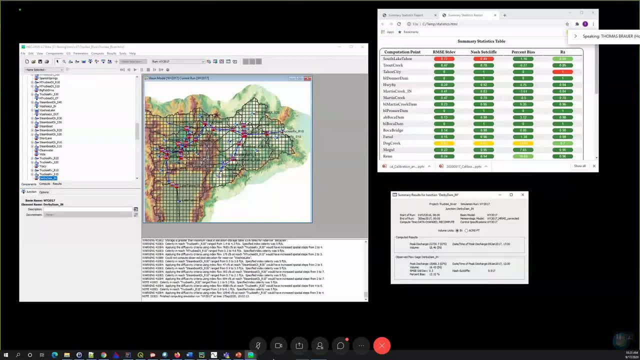 especially because often around our biggest events, the data quality is the worst. um, maybe because the you know the stressing the instruments- i've seen it time and time again- where the biggest flows on record completely wipe out all the discharge gauges, which is just like for us who are modeling in this high flow world. you know, you say doing damn damn studies. that's the. 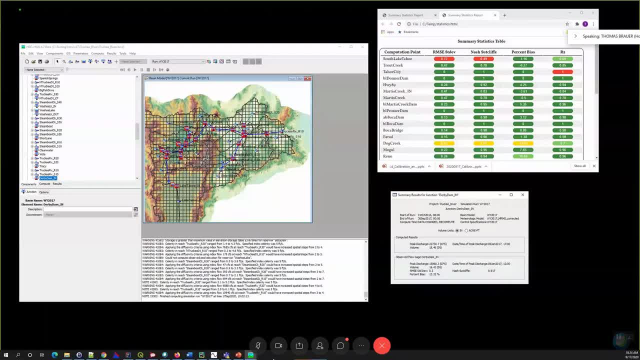 data we need and the gauges just wash downstream, you know, and so for the most critical part of our analysis, we don't have any data. so, yeah, it's really hard to say that's a good question. i'm going to say it's really hard and it's um, it's difficult to go through. so you have five events and like four of 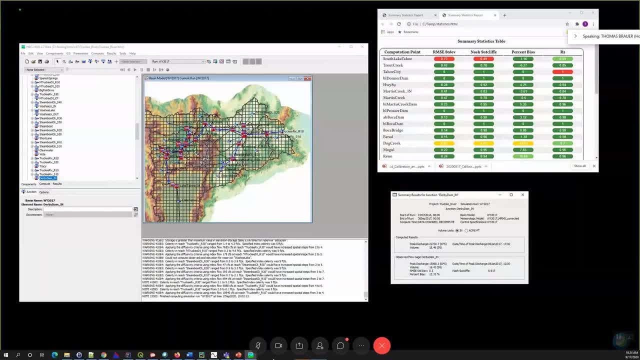 them are are medium high and then that really high one. you have a high one- i precip high flow event and the data is bad on it. so it's hard to to pull that um. you can massage the data. you can say, hey, we, you know, looked at this and we did this. but the biggest thing, if you start so, one option is just to 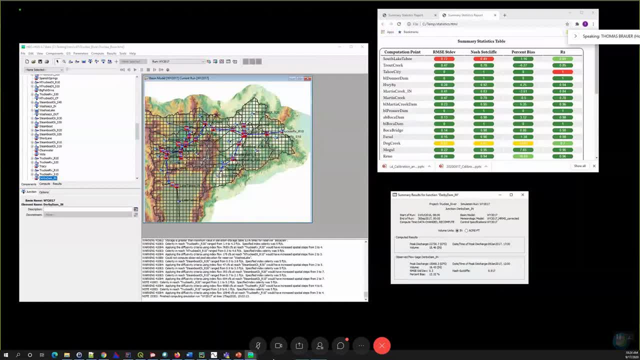 throw it out and not use it. the other option is to massage it. the only caveat i give with massaging data is: just be sure you can back up what you're doing and have really good reason for it. i know i've had to do that on a continuous study. we had to go in and reevaluate the volume for 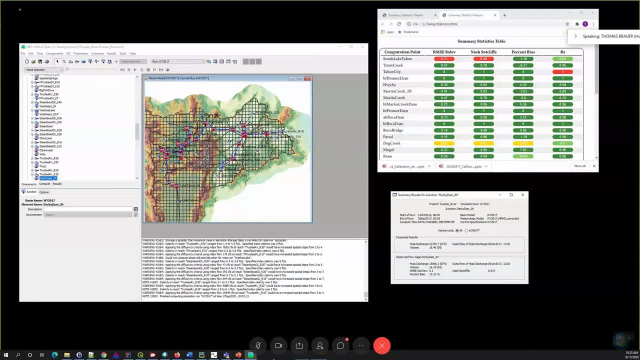 the biggest event on record, which is the. i was doing modeling in the russian river, and the biggest event on record was 1964. event data in 1964 is not great, um. so yeah, we, we looked around at neighboring gauges, figured out what they were doing um things like that, and justified 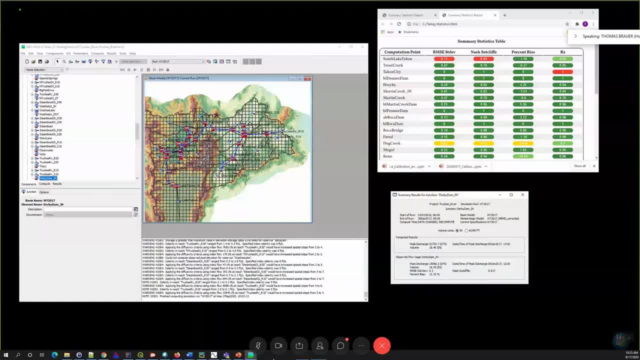 what we did, but that's just the caveat. you can, you can try to massage it, but you just definitely um put it in your report, talk about it, all right. um, just a couple more here. um, we have a question about how grids are created for this model. it's probably too much to cover on this particular call, but 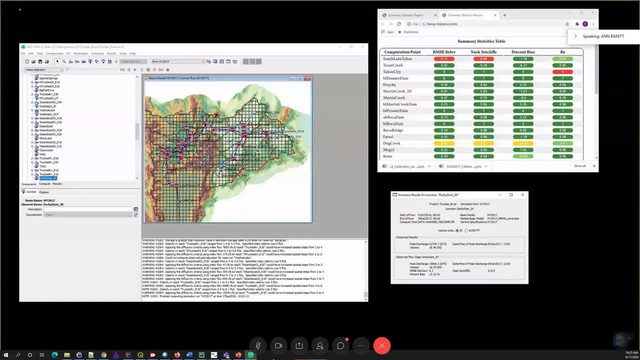 it's been a lot of fun and i think it's gonna be interesting to hear more about that. yeah, absolutely. um, so i'll just- uh, i'll just kind of cover or just mention how etc's posting some of your training workshops, that sort of thing. so if people wanted to learn more, if they haven't had the 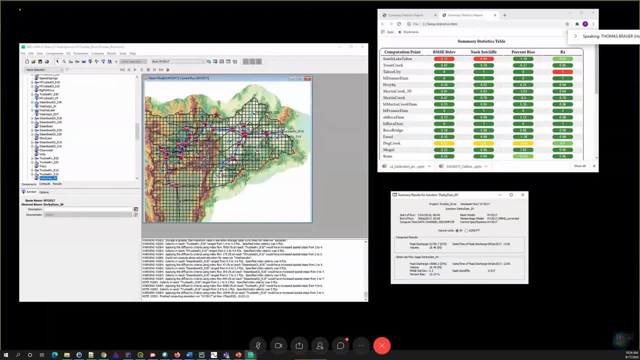 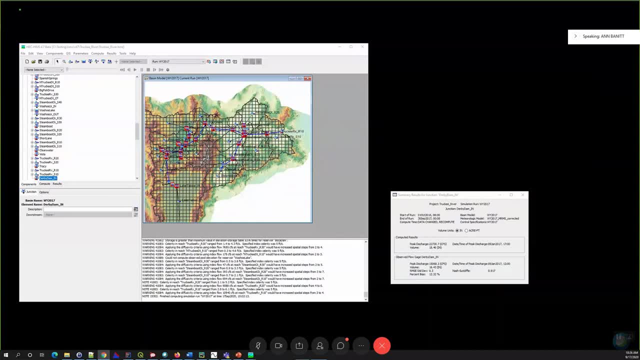 internet class, yet we had one delayed, okay. so the questions about how the graded boundary conditions are created, is that right? and then you're you, you suggesting that i pull up just like our training material. yeah, but i was, i was thinking just kind of okay, yeah, yeah. 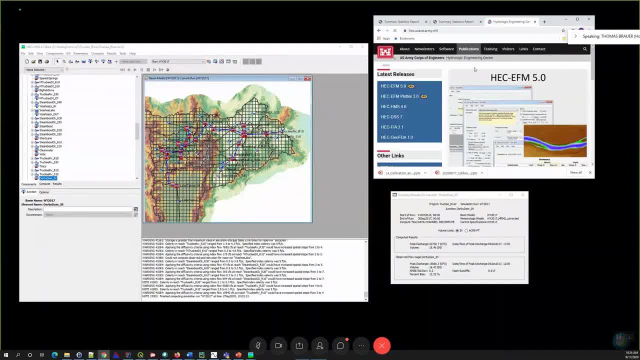 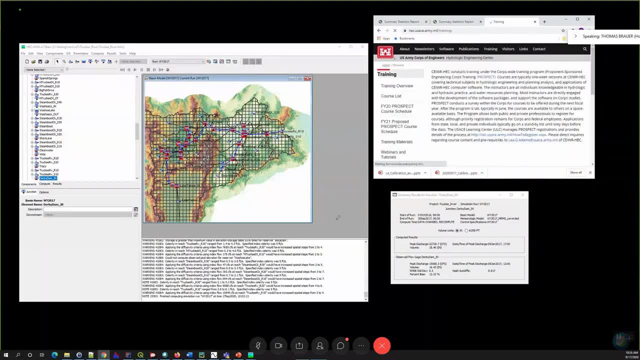 I can address the question. It might be a little out of scope, but it's a good question. Let's take a look at the training though. So yeah, we've done a lot of work in the recent past to put our training material on time. 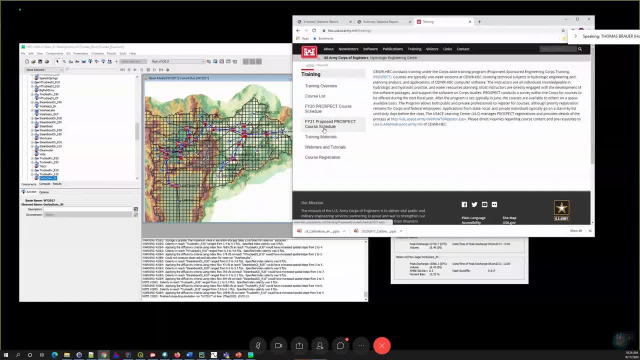 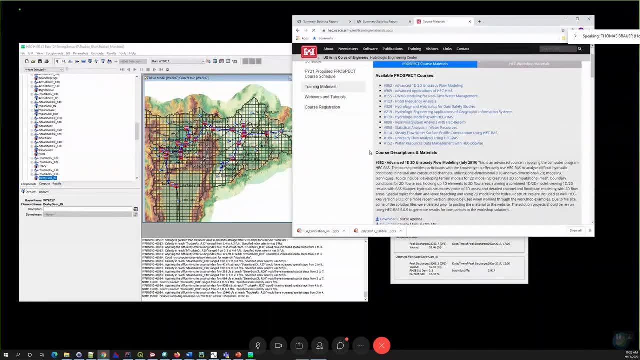 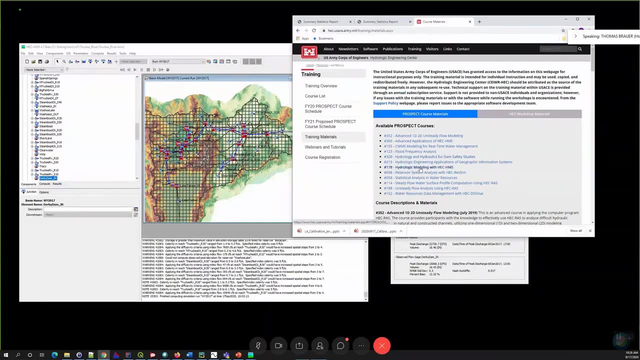 So if you haven't attended one of our courses recently, let's see Training materials. So I'm just on the HCC website Training materials And here's our – we put the entire prospect courses online And so I would take a look at – there's 178 is our basic class. 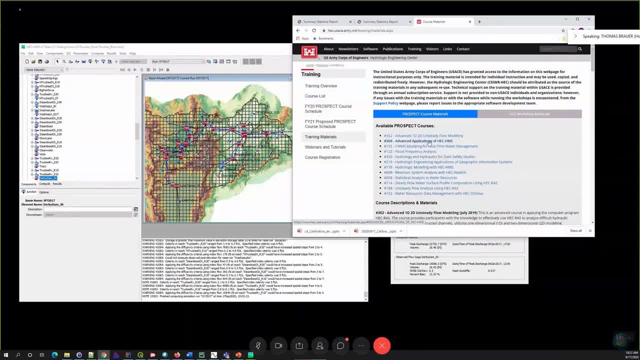 There should be a 369 on here, which is our advanced class. that has all the training materials, And then next FY. we're trying to do more and more digital online training, Like hopefully this presentation gets pulled into a video and we post it and it's there for everyone for all time. 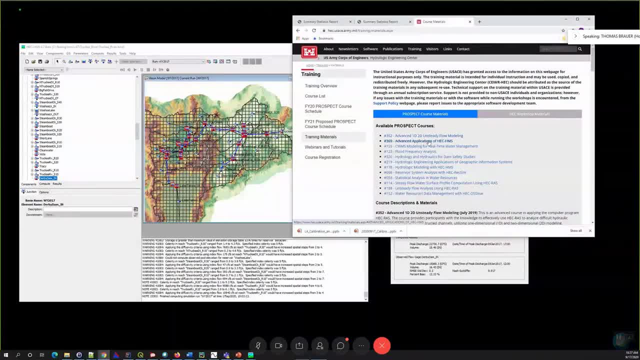 But we're hoping to do more of that with our training classes so you actually have like video and audio as well. So do you want me to talk to that question? Are there others I can talk to it if you want. Yeah, I think we're kind of at the end of our window. 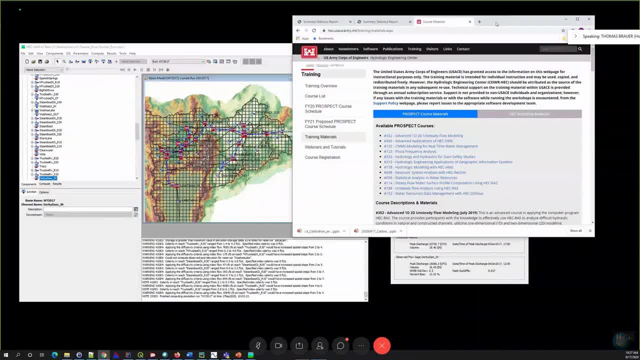 Okay, Maybe we'll discuss between our POCs and our division if that would be a valuable separate webinar. I think that's a little bit more than we could in a couple minutes, But maybe highlighting where you'd look for the gridded training. 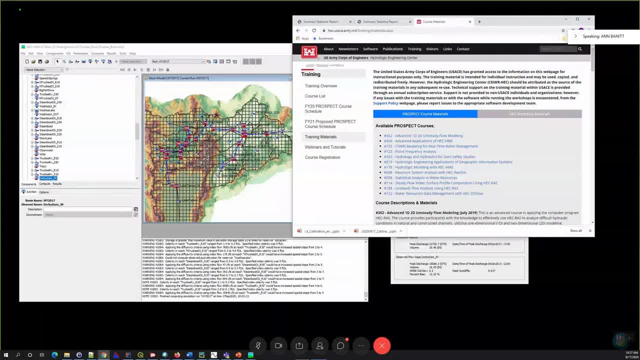 Is that in your basic HMS class or is that in advanced? The advanced, I know, has a gridded section. Yeah, I believe the advanced has a little discussion of gridded modeling methods. If they're talking modeling methods, there's probably some discussion there.